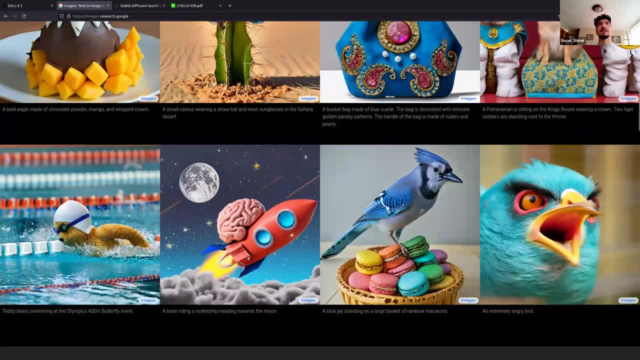 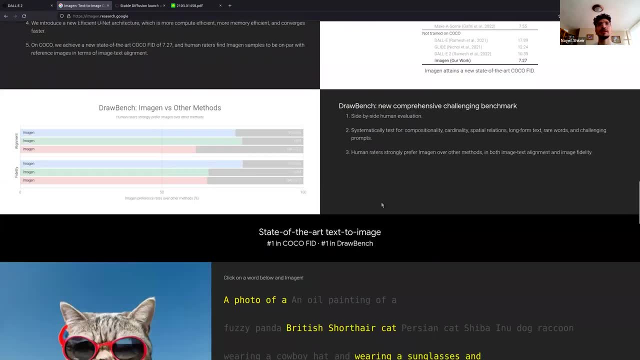 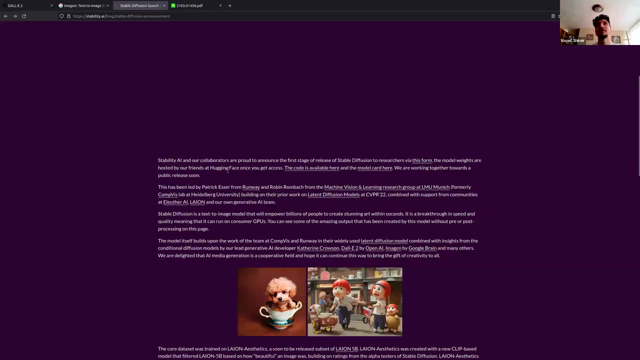 did sort of image generation from text And they did super resolution using diffusion models And I think it was something, yes, like text to image And yeah. so this is like super interesting work from them. And then like there's other groups from Stableai- This is pretty recent, I think, Yeah, still. 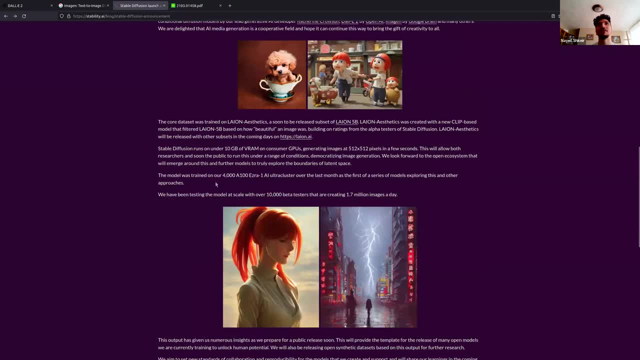 like a couple of months ago And again, sort of they were doing image generation from text And then I sort of was going a little bit through the literature on diffusion models and what work has been done, And then I thought this was really cool, where you can generate. 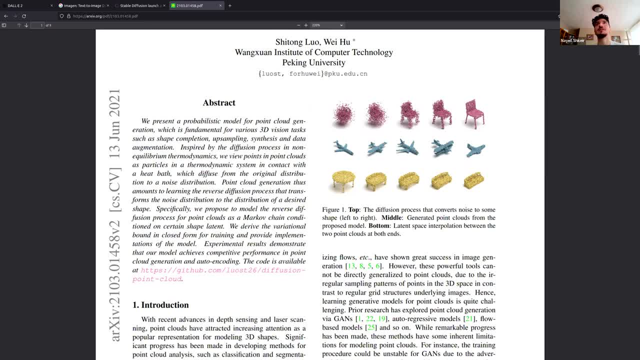 objects from sort of point clouds, And so this is a sort of 3D isotropic Gaussian, And so from this 3D isotropic Gaussian you sort of generate a chair, which I thought was really cool, And it sort of uses the whole theory of diffusion models to do this. But yeah, Okay, so let 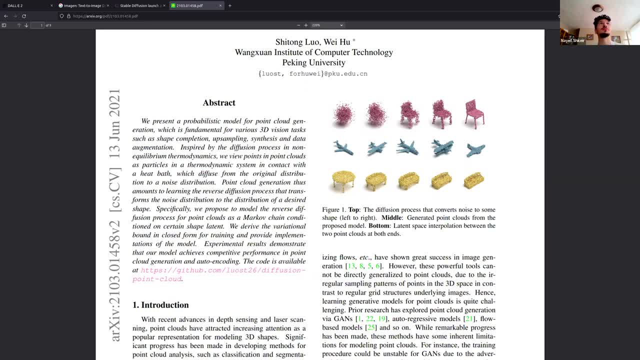 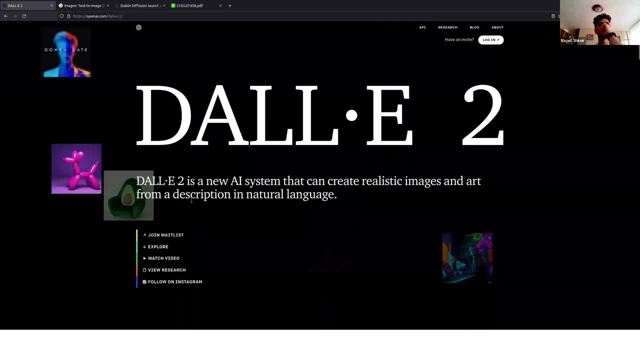 me actually go to the paper And this is like super fun to play around with. So, like I'd highly recommend to like mess around with this, And I think they have a- Yeah, they have a- wait list where you can do like beta tests on their model and so on, But yeah, 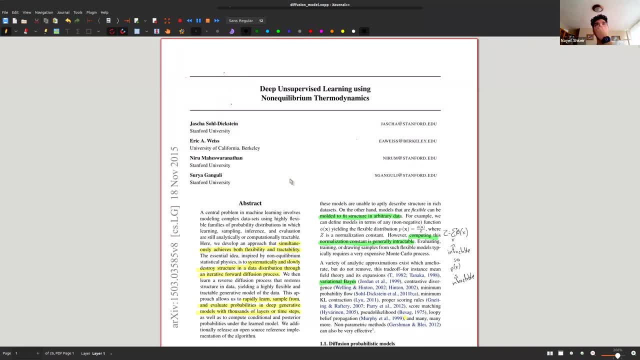 anyway. Okay, so this is the paper. So the paper that sort of started this whole diffusion model field, I guess in generative modeling is this sort of deep unsupervised learning using non-equilibrium thermodynamics, And so this is a really fundamental paper in diffusion. 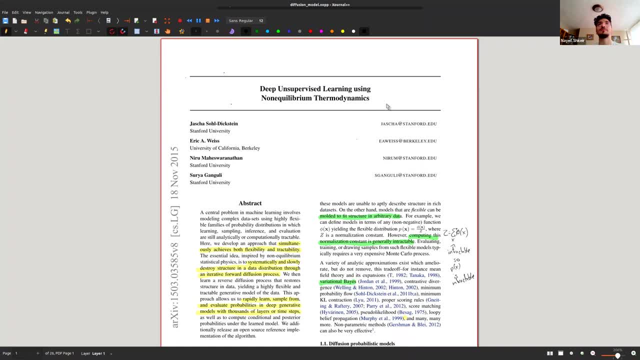 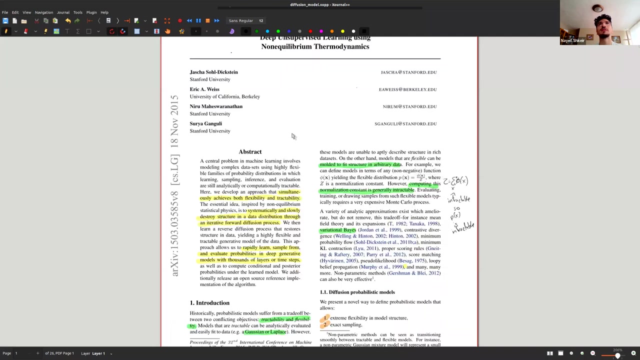 models And it was sort of the first one to really introduce them. Yeah, so it's very fundamental, But it's It's pretty important to get into diffusion models with this paper first, Because it sort of It helps build a foundation on it. So this is a paper by a group at Stanford where they 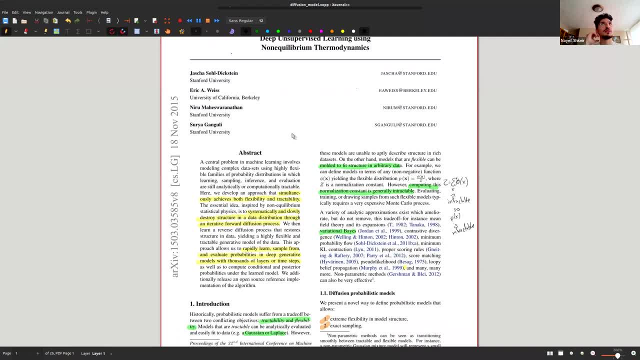 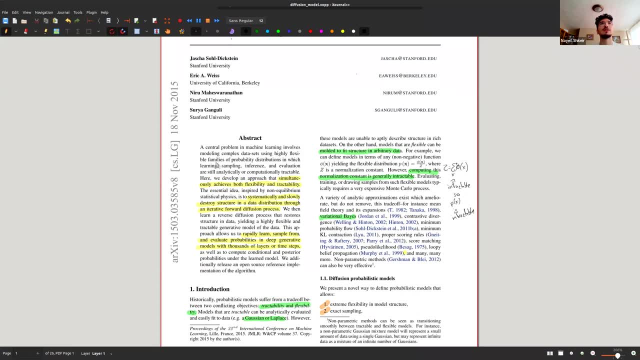 sort of try to use this statistical physics and thermodynamics for their model, for their generative model, And so in this paper so they develop an approach that simultaneously achieves both flexibility and tractability, And so the whole sort of In this diffusion model you take some sort 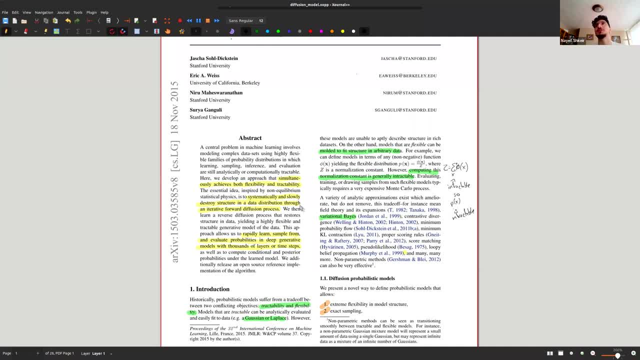 of image or whatever data you have, and you sort of destroy any structure in this data through some sort of diffusion process and then you reverse it And then sort of they go into sort of learning, sampling and evaluating probabilities from this generative model. 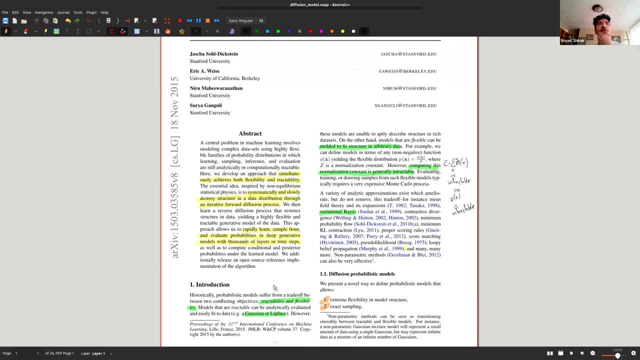 But yeah, okay, So in the introduction. so they say Okay. so probabilistic models suffer from two main things, So tractability and flexibility. So a lot of the distributions that you're going to be working with in generative models are not really tractable unless sort of you're working. 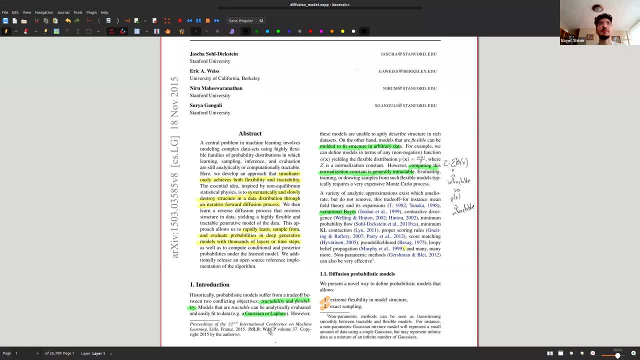 with Gaussians which are sort of super nice. And the other main thing is flexibility. So can your generative models sort of generalize to any arbitrary data, Or can it sort of generate data from sort of a, A geocache, a big sort of distribution? and those are the sort of the two main. 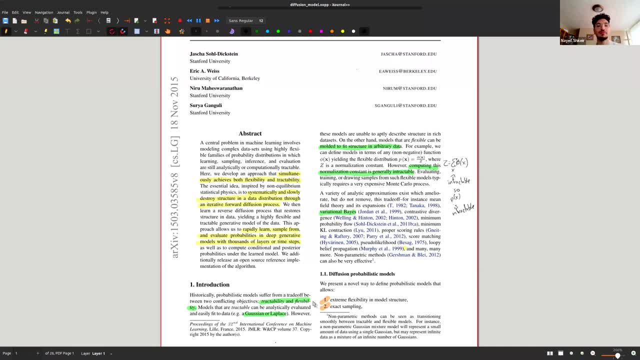 like problems that these generative models try to solve and sort of these are the main problems with them, and so this paper tries to address both of them. and i think they pretty much do, uh, and they do it pretty nicely, and so then they also say so, for example, we can: 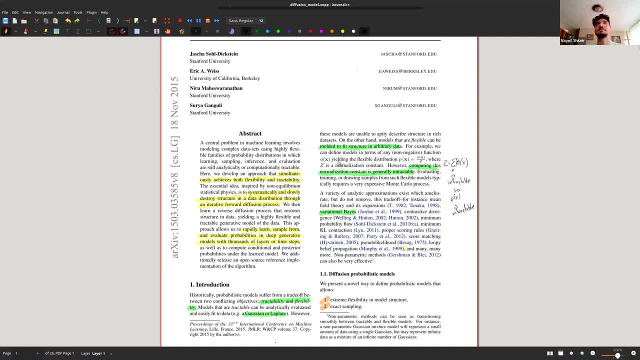 define models in terms of any non-negative function, phi, yielding a flexible distribution where sort of you have a normalization and this sort of normalization, it's just the sum of x over x, which is of a 5x which is intractable. uh, so then the distribution of x is also going to be. 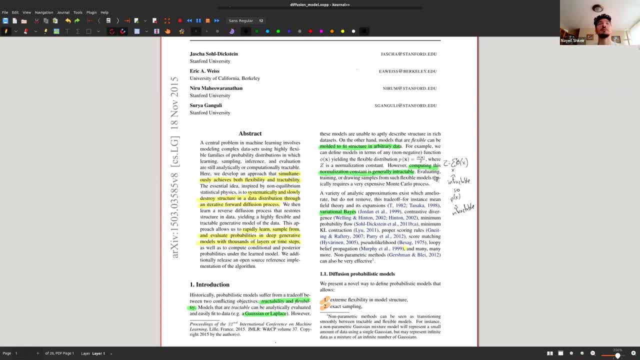 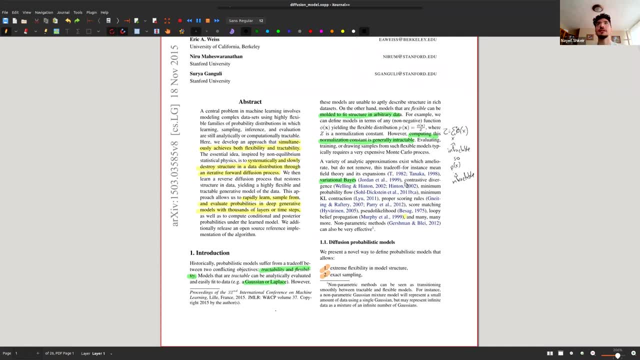 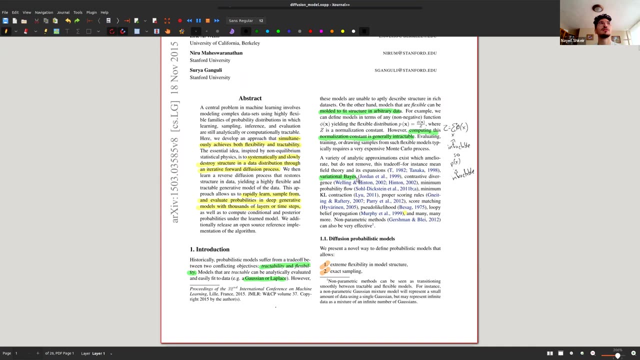 intractable uh and so, but they show that using this, uh, diffusion model, this is actually pretty easy to do. um, yeah, and so they have. so they show like variational base. so this is pretty similar to auto encoding variational base. uh, the algorithm, uh, for variational encoders, uh, the ideas are sort of 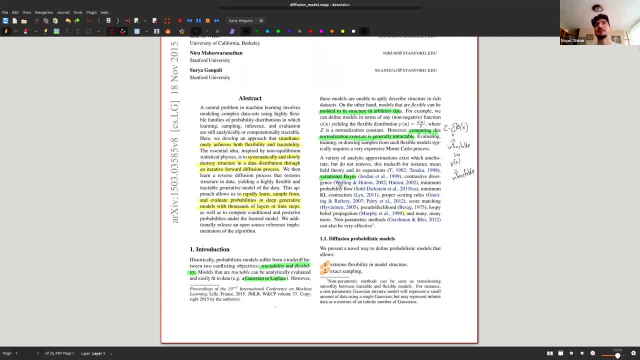 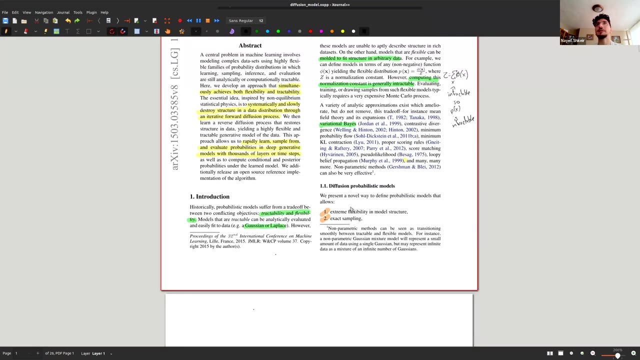 uh, pretty similar and so the derivations are similar, uh, but yeah, so that's sort of a main part and sort of yeah, so there are other methods that sort of try to sort of solve this tractability and flexibility problem in generative models. but yeah, so in this, so the diffusion probably models, that's what they call. 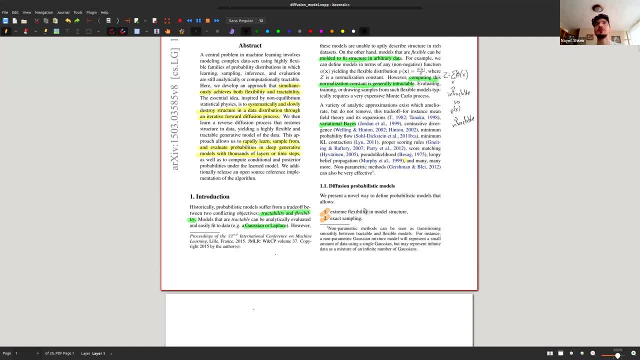 the model that they present here. so they define a probabilistic model that allows them to sort of have extreme flexibility. model structure right, they can generalize a lot of different uh data distributions. so you do exact sampling which i think will make sense once we go into the actual model a bit later. 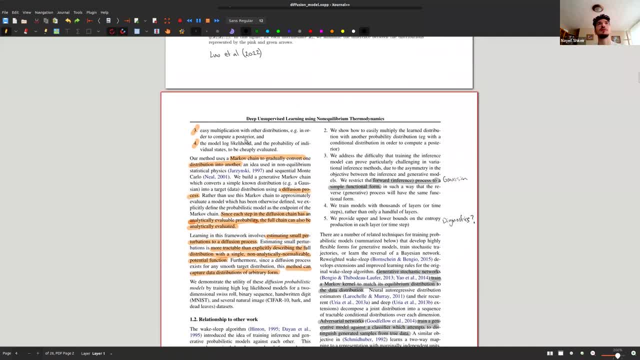 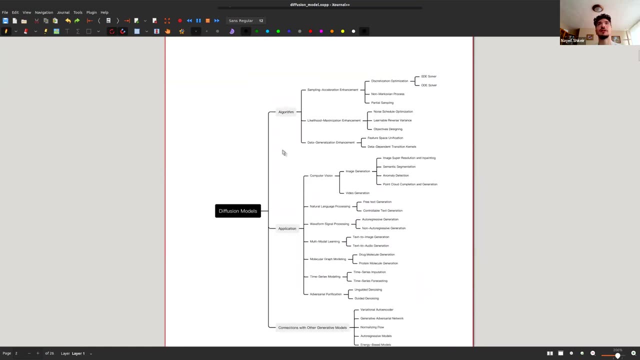 um and wait. so i did some stuff there and okay, so easy multiplication with other distributions and you can compute the model likelihood and the probability of individual states cheaply, okay, so i think. so i put this sort of diagram here as well to show where diffusion models have been used. uh, so in sort of application wise of diffusion models. 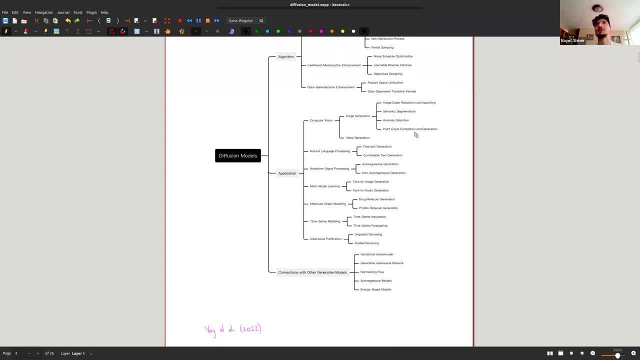 in computer vision you can do image generation, so super resolution, uh point, cloud, uh generation, which is what i showed with the 3d models, video generation and in text, sort of free text generation, also generation with um signals, um drug generation, molecule time series, so yeah, so there's loads of different. 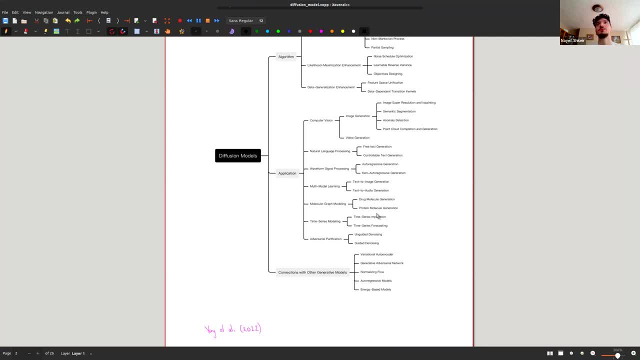 applications for this and the main competitors with the diffusion models are sort of the vaes, the general adversarial networks, normalizing flows and auto-aggressive models. uh, so yeah, so there's a huge field of application for these sort of models which make them sort of really interesting. they're able to sort of work with so much different types. 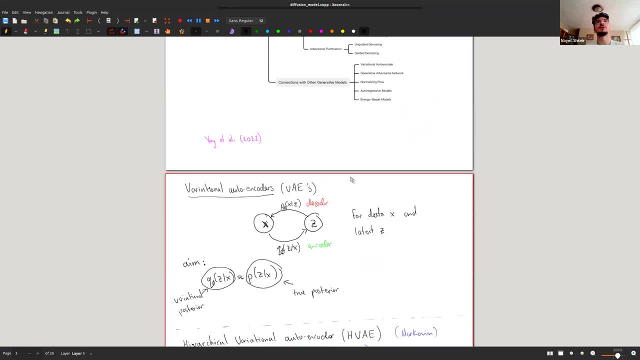 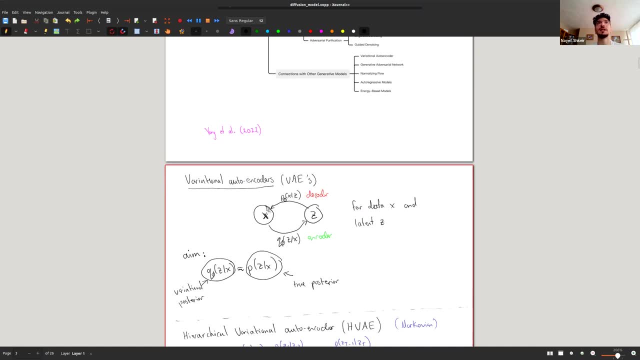 of data, yeah, so before we get into the actual model. so i thought it would be good to have maybe a little bit of fresh air into variational encoders. so with the version of variational auto encoder, you have your data x and some latent zed and so, um, you're trying to encode the information from x into some. 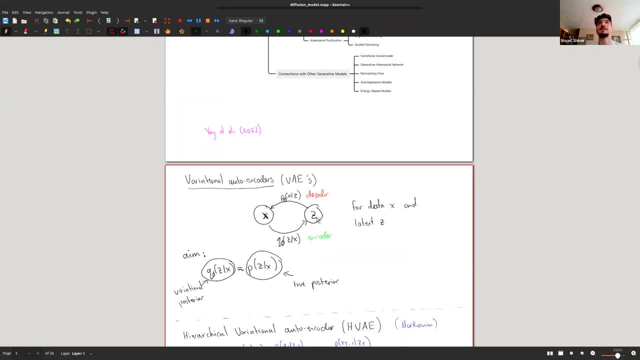 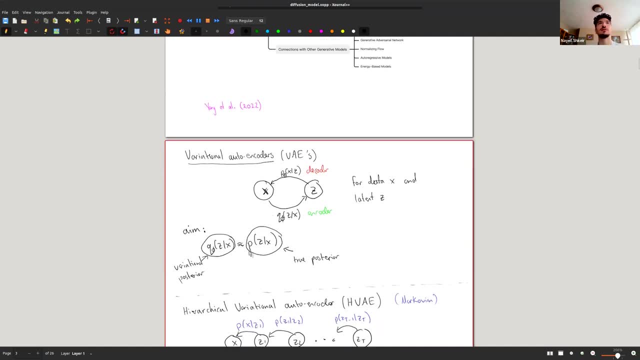 latent zed using a encoder and then you sort of try to decode this information um back to x, and so the aim is to sort of have the very close to the true posterior as close as possible to the true posterior. uh, for some data x and latent. 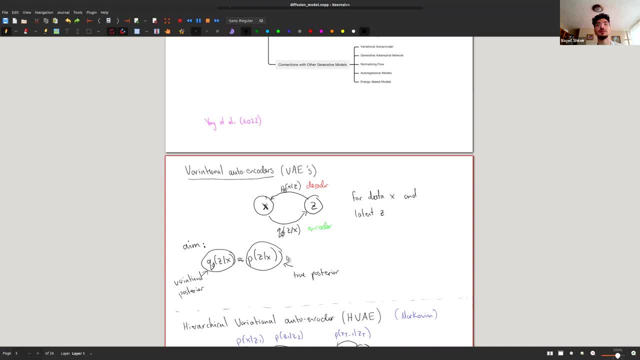 zed right. so you have a neural network that will sort of compress your data into lower dimensional z and then you'll sort of upscale it back into x and uh. do the uh- the difference in distributions, and then you're trying to minimize that. so these are sort of variational auto encoders. 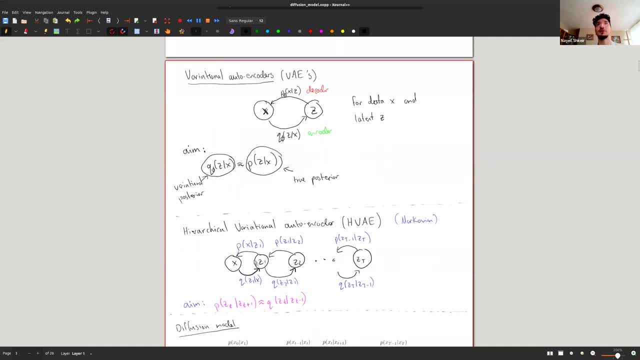 and there's an a generalization of variational auto encoders, which is hierarchical variational auto encoders but specifically sort of uh marco, so as in the next state is only dependent on its previous state and no other state before it. so you take your uh data x and you sort of encode. 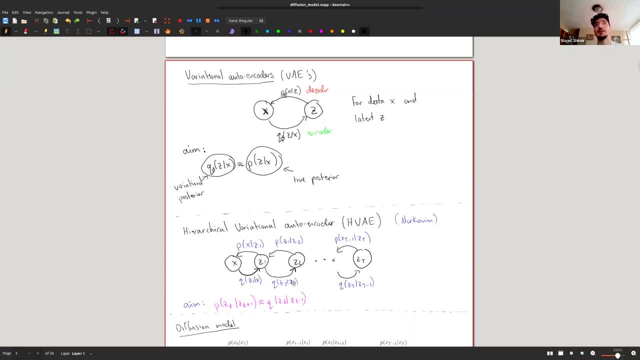 it into some latent z1 and then you encode that latent z1 and turn up the z2 and so on, until some t, which is a t, is here like a layer in your, in your network, so like how many layers you have here- and then you again have your sort of decoder part, uh, just like in the ve, and again so the 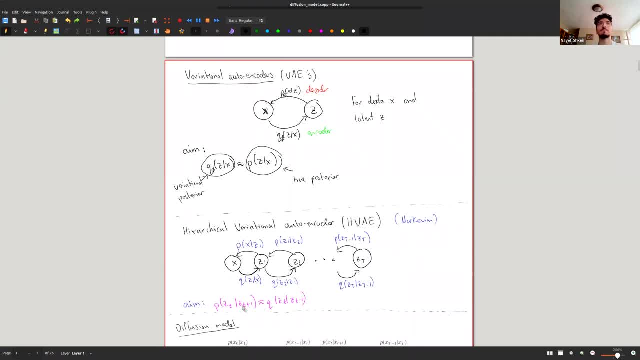 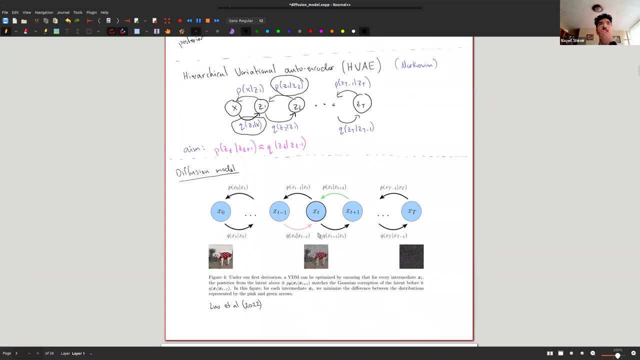 aim here would be to um match, uh the posterior of uh sort of this encoder to that right. so you sort of you'll be trying to sort of minimize this, uh, this difference in distributions. uh, so okay, so models are an instance of hierarchical variational auto encoders. so okay, so this is um sort of the. 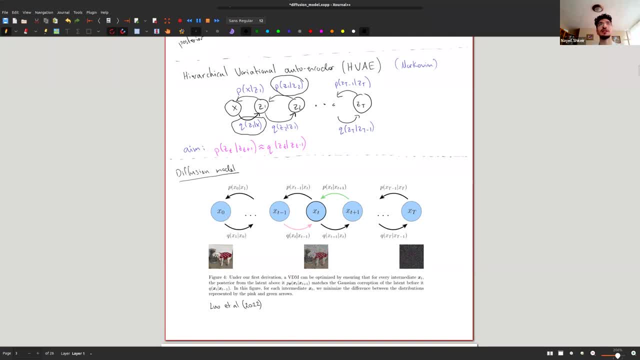 main idea of a diffusion model is: you take here, you take an image x and you push it through some uh, into some latent z, and then again, and you keep doing that, and then you keep doing that t times until what you have left at the end is, um, just pure gaussian. 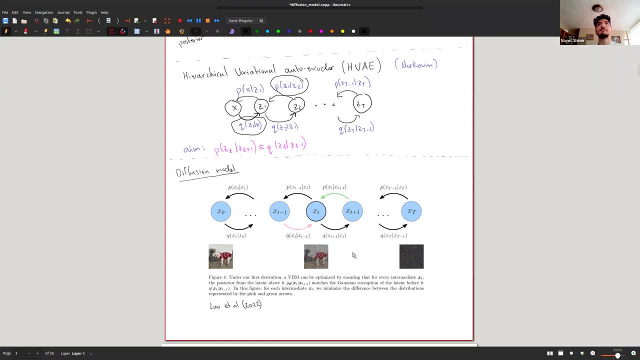 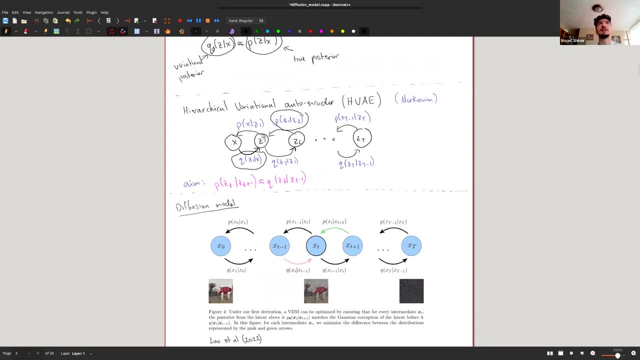 and the reason why this is an instance of the hierarchical variational encoder is because, well, in the auto, in the hvae, the latent zeds are going to be of sort of lower dimension than your x's, whereas in the diffusion model your x and zeds are going to be of the same dimension. 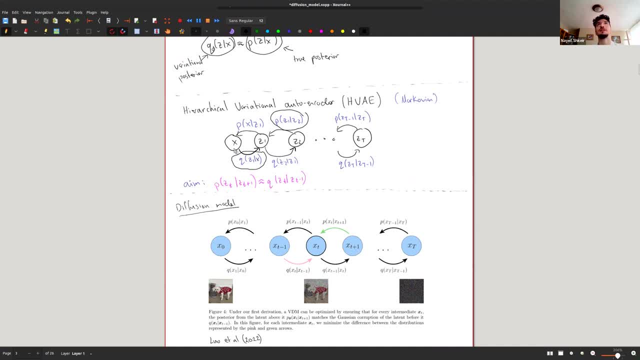 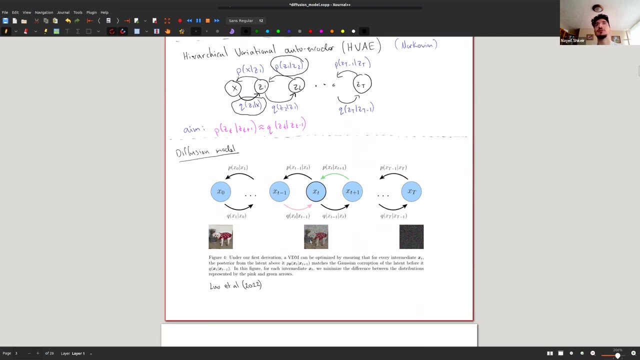 um, and the other thing is sort of the encoding process is fully defined in the future models which will make sense a bit later. but yeah, so the sort of a nice example here is you go from this image of a dog and then you keep adding sort of gaussian noise until sort of becomes blurry and 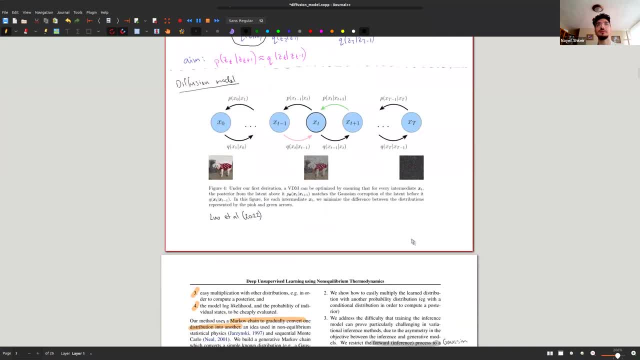 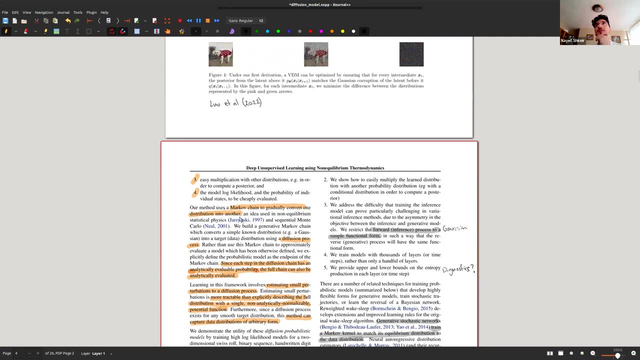 then becomes fully, uh, just full noise. but yeah, so so this one says so. our method uses the mark of chain to gradually convert one distribution into into the other. so you're converting this distribution of an image of a dog into just noise, so using the idea of non-equilibrium statistical physics. so they mentioned this. 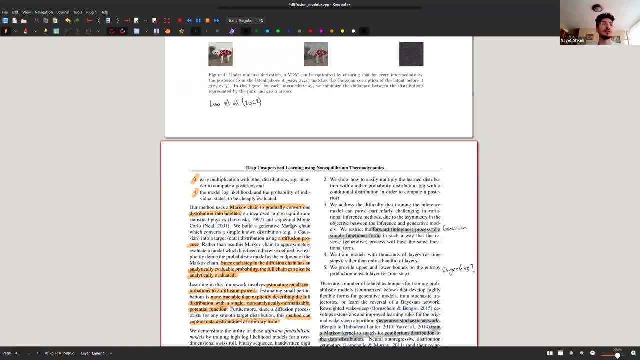 quasi-static uh idea from thermodynamics and i guess how i understand it is. so if you imagine a box with a lot of gas inside that's at equilibrium, so that's at an equilibrated sort of uh pressure, then if you take the boundary of this box and sort of decrease the volume, just 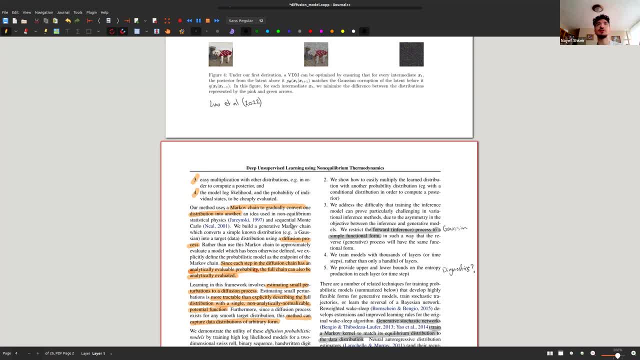 a tiny amount but it doesn't cause a big disruption, such that you have sort of like an instantaneous adjustment to uh equilibrium, and so that's this sort of quasi-static equilibrium, where you can sort of change the boundary or something, but you're still in equilibrium uh. so that's sort of the main idea that you use from non-equilibrium thermodynamics. 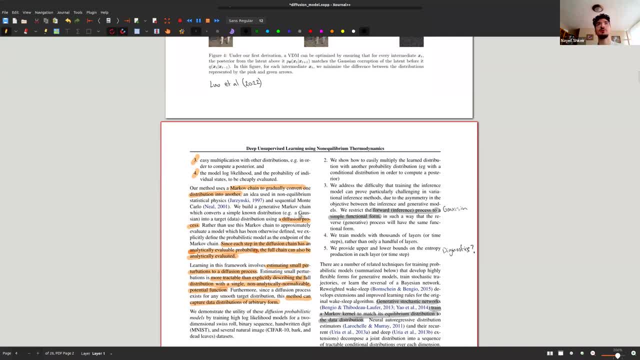 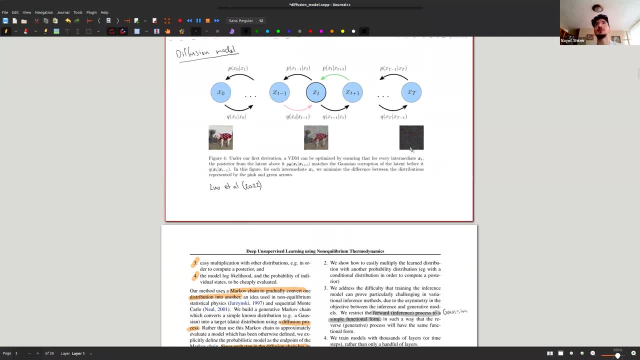 uh, yeah. and so they build a generative mark of chain which converts a simple non-distribution into a target data distribution. and so you go from. you could take your image, you convert it into a gaussian, nice gaussian, yeah, is that? one impression i got from the model that they're using is that they kind of assume that. 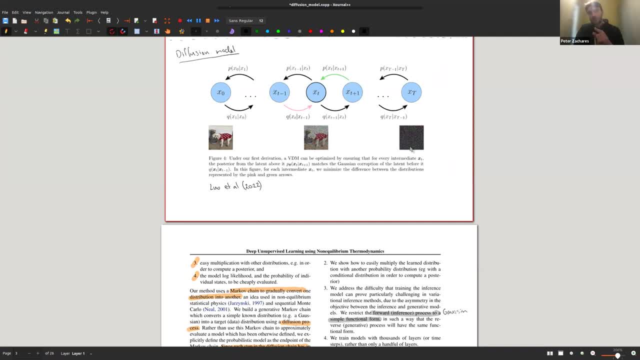 between steps in the diffusion process, there's only very small changes. yes, with this quasi-static assumption, yeah, exactly that's why. so like, like in the box example, like you decrease the volume of the box a tiny amount so that you're still in equilibrium, and here you do, it's like a tiny you. 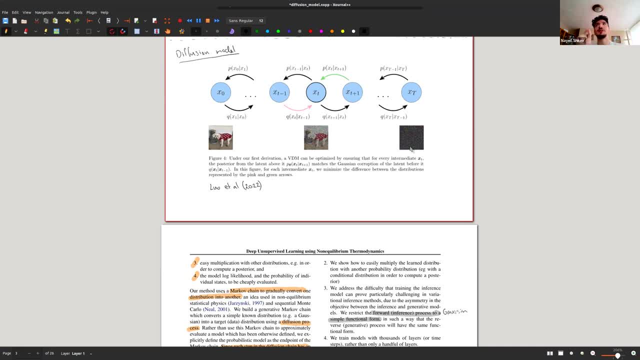 add sort of tiny gaussian noise such that your whole model doesn't break down, so that you still get to retain some information. because if you just add sort of like, if you go from one image and add a huge amount of noise, then sort of you haven't really learned much. 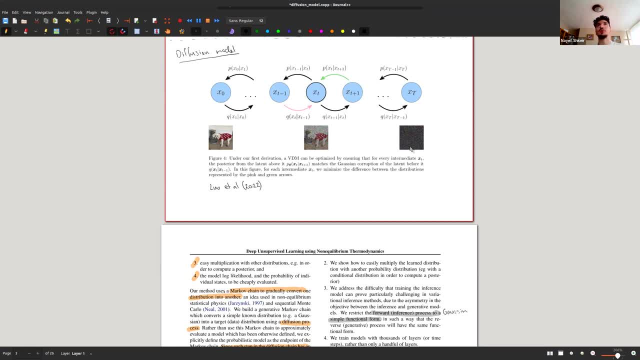 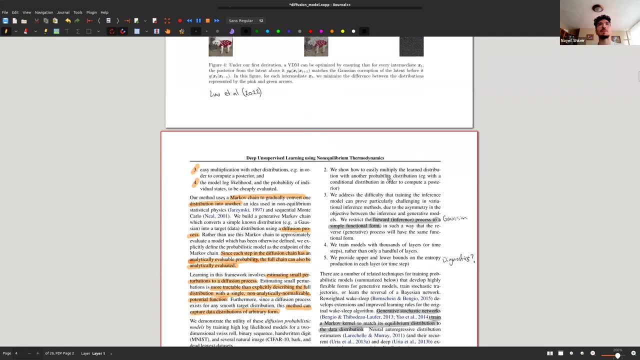 like you get rid of data or sort of structuring your data way too quickly, so it has to be sort of really, uh, sort of small steps and a lot of these steps. yeah, that's where i was struggling a bit, right? so if we have two images as input, 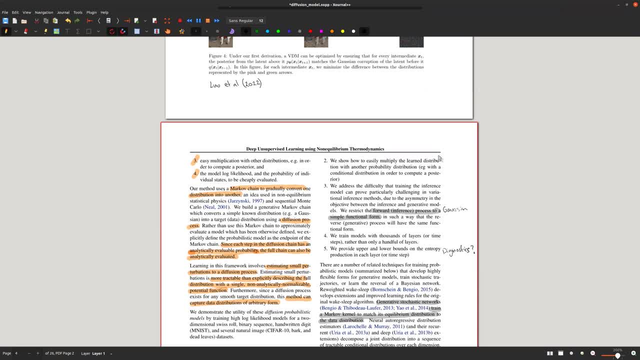 and the at the very end in the encoding layer. essentially they are, as you said, isotropic, gaussian. yeah, how can we possibly reconstruct two images from noise? yeah, that's a really cool part about about this, i guess, and it's it's all to do with, i guess, the reversibility in this diffusion process. 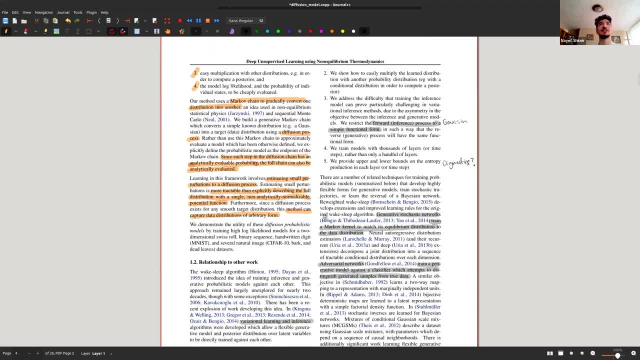 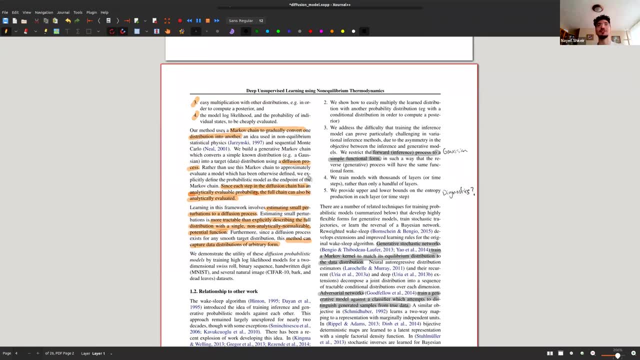 which is really nice. um, yeah, which, yeah. so i think i have something where i'll mention about sort of some stuff about reversibility, but yeah, the whole idea is a bit crazy, where you can just take noise and reconstruct something that makes sense out of it. but yeah, uh, yeah. so, rather than use this market change, so approximately evaluate the model. 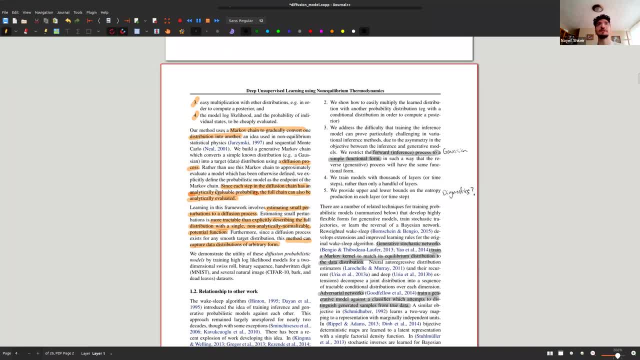 we explicitly define some properties model as an endpoint of the markov chain and so each step in the diffusion chain has an analytically evaluable probability. so the full chain can also be an analytically evaluated. so that's a really powerful property, i think. 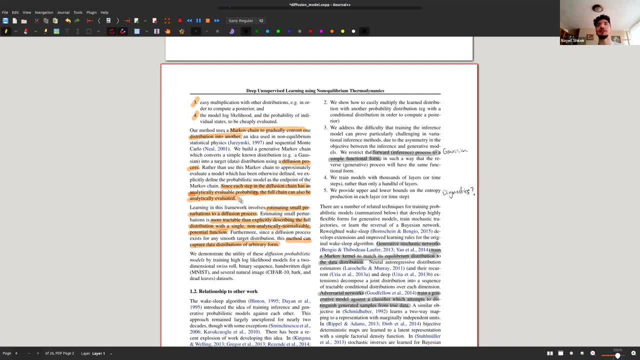 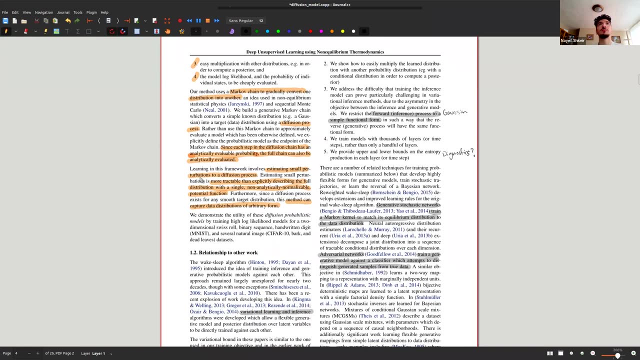 because, well, the diffusion pro, you're the, so each step, you, it's fully defined right, you have some parameter and it's just a gaussian right. so you, you can, you have the full form, so you have the analytical form, and so learning this framework involves estimating small perturbations to a diffusion process. 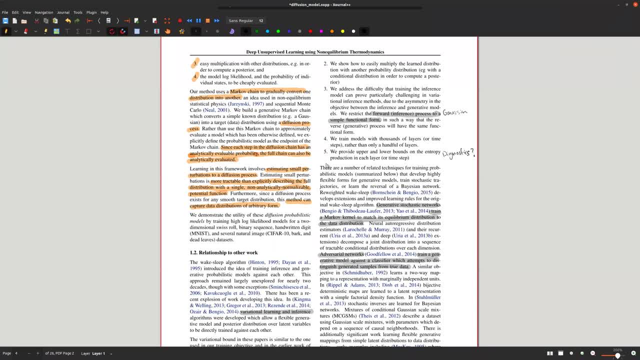 when you say you have the full form, is that the the kernel of the diffusion, that that's the yeah, um and so yeah. so estimating small perturbations more attractive than explicitly describing the full distribution with a single, non-analytically normalizing potential function. so i guess the way that i understood this is sort of it's much easier. 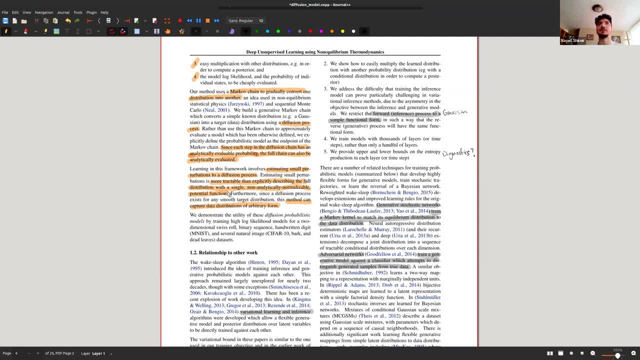 to work with sort of small changes to something than sort of just a big, like a big change in your data. yeah, and so this method can capture data distributions of any form? i didn't. i was still thinking about what they meant by, since a diffusion process exists for any specific. 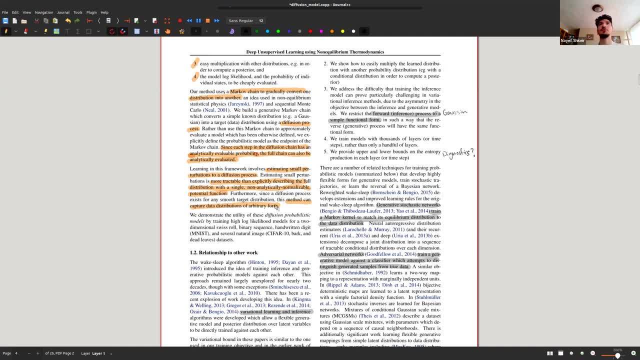 the target distribution. i was thinking sort of what are non-smooth target distributions, but i i don't. i couldn't really think of any. like a rectified distribution, for example, would be non-smooth, right or no, yeah, but um or maybe not. it just, it's just like it's support ends at zero. 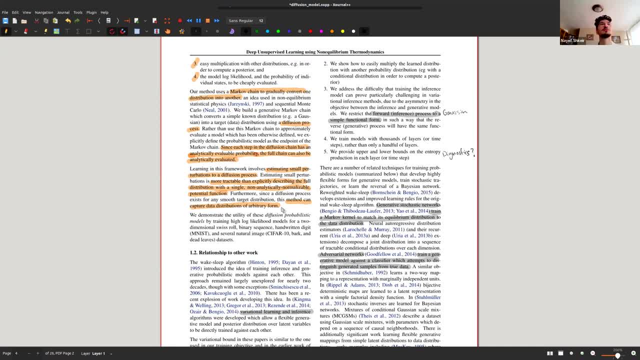 that would be a rectified distribution, yeah then. yeah, i was thinking like how a diffusion process would sort of struggle for something like that, but maybe, maybe, if you were to have like, uh, i think, um, i guess re it would. yeah, this is an obvious one- is like regions where 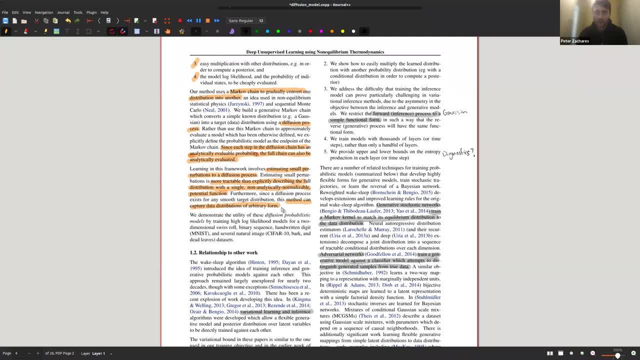 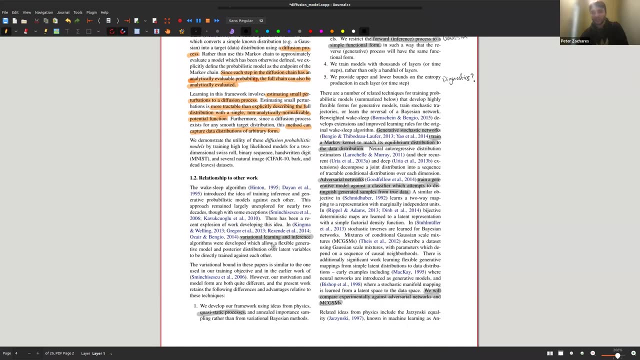 where it's possible to have a value, in regions where it's not possible to have a value in the. in a continuous, that's true, yeah, in a continuous distribution. yeah, yeah, actually, yeah, that's true, uh, okay. question: uh, is diffusion a stochastic process? uh, yes, okay, yeah, so it's sort of browning. 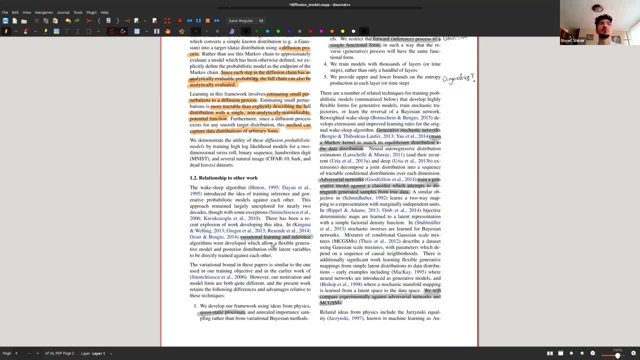 motion if- if you sort of done that before, so it's like um, or like a random walk where you sort of you are at a position and then you just add some sort of- uh, normal gaussian to sort of take you to another, uh step in some area around you, so you just randomly move in some space. 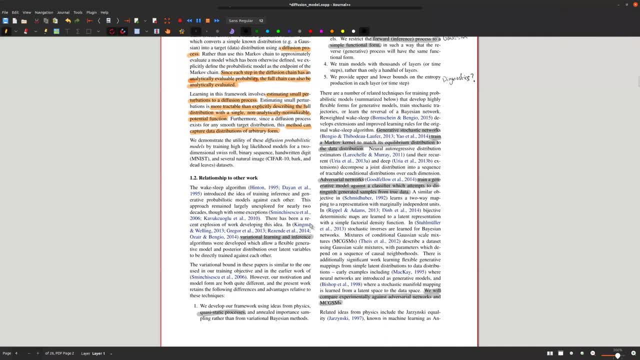 and isn't. when you apply diffusion, right, you, the, your general process, uh, inequality holds, uh that your, your entropy always is increasing, right? yes, so so when they say that the reverse process is also diffusion, wouldn't then that say also that every step they increase the, the entropy of the 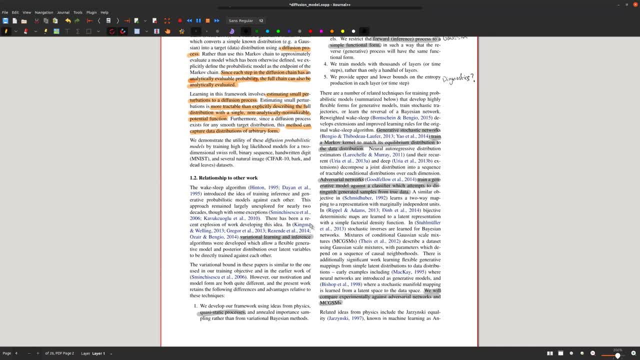 solution, and and how do they still come up with something that that looks not like even more? and also because generally it's, it's a lot of these things you, you can, you can't really diffuse backwards in time in in in regular physics, right. so when you, yeah, you can, you can, you know, play a. 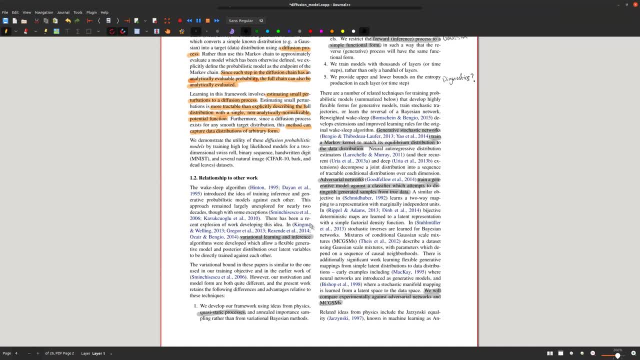 move backward, but but in reality, because, because it's adding sort of noise, it leads to the same state of, of of your, your particles, being being distributed. now it's, yeah, it's, i guess, yeah, i guess. the way that i think, i think of it is more sort of a sort of an in a dynamical. 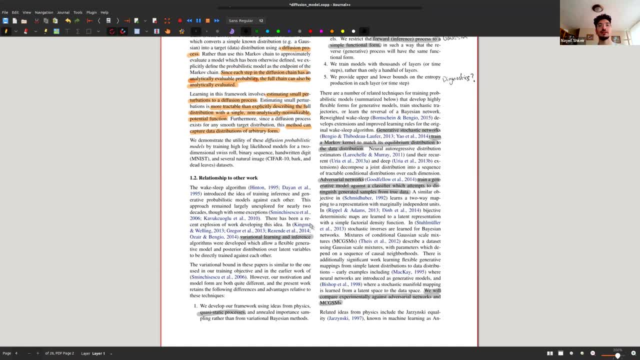 system point of view, it was like you'd have a path from your data to some um, from your distribution, to sort of an isotropic gaussian. so it you apply some sort of um, you applied some dynamics a long time so to evolve that path to the isotropic gaussian, and then 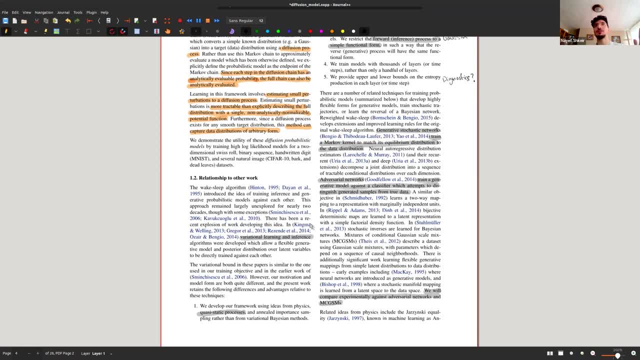 because of the, the properties of sort of diffusion, you can retrace that path back and sort of you learn that the path back and sort of you can retrace that path back and sort of you learn that the path that you took and sort of space, uh, to your isotropic action. but yeah, yeah it's, it's pretty. 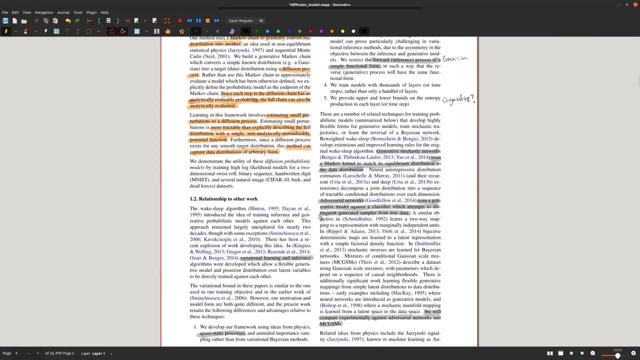 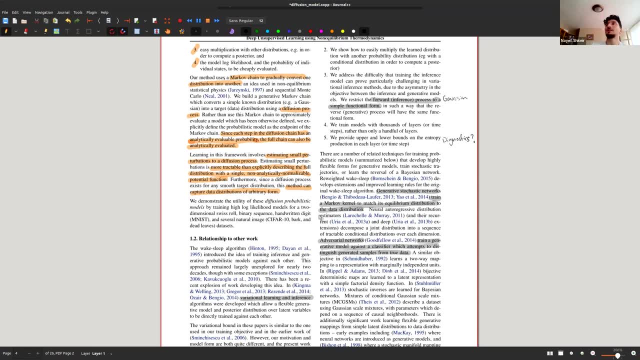 confusing to get your head. the diffusion concept itself must then be a function of time, right, the? the diffusion kind of can't be along your path. yeah, so you have some mean that's sort of uh prescribed, that sort of pushes you to some sort of um point in your space. 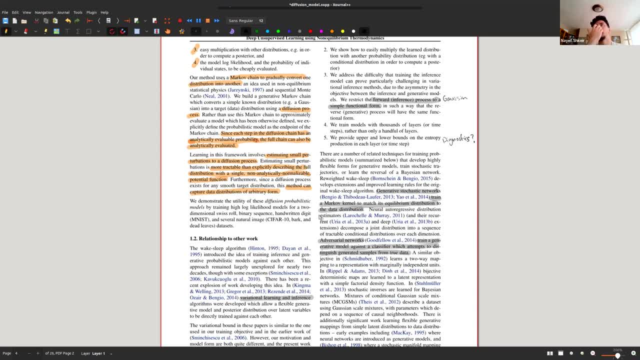 okay, just sort of like drifts you to a certain point which is: so it's not really a diffusion, right, so it's not like your diffusion, no, no, yeah, so you have like a sort of sink somewhere in your, in your, yeah, then then it sort of works then. then then you sort of reduce entropy by doing that it's. 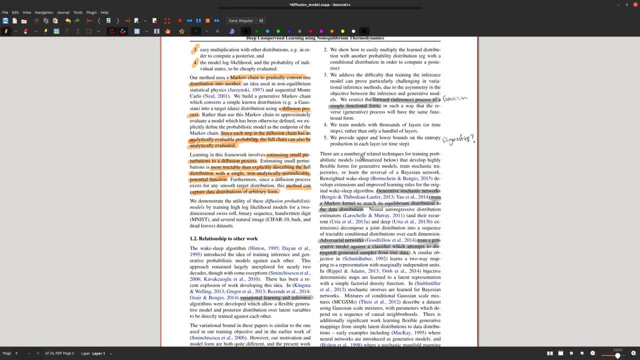 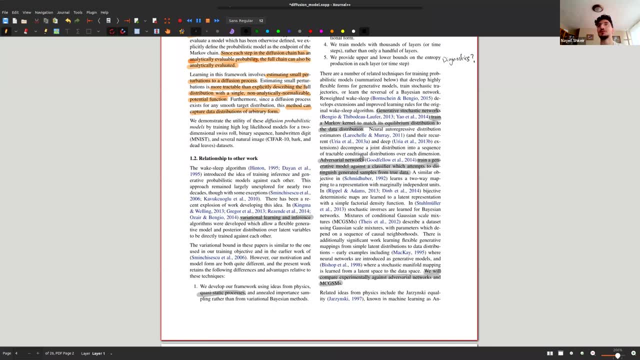 like a fridge right where you know, no matter where you end up, you end up being cold. yeah, yeah, yeah, i guess. yeah, that's the a really important point. it's like you have your random sort of walk, but then you you're also tended like you walk randomly but you also tend to go in some certain 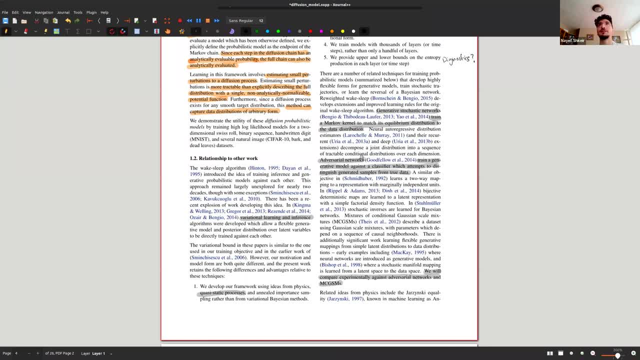 position into a certain direction by sort of the mean that you have but yeah so, yeah, so there is some work before that was done. so the main- i think the main competitor i would, i would guess- for these sort of networks is sort of gans, just general adversarial. 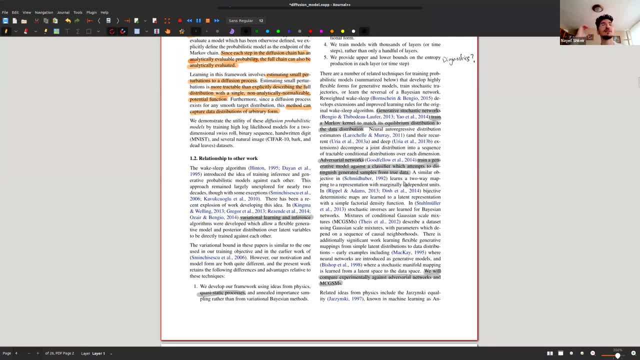 networks by sort of goodfellow, which i think he was. he also helped with this paper, uh, but yeah so, where they train a generative model and so on, and so they compare a little the results that they have here against generative adversarial networks and these. 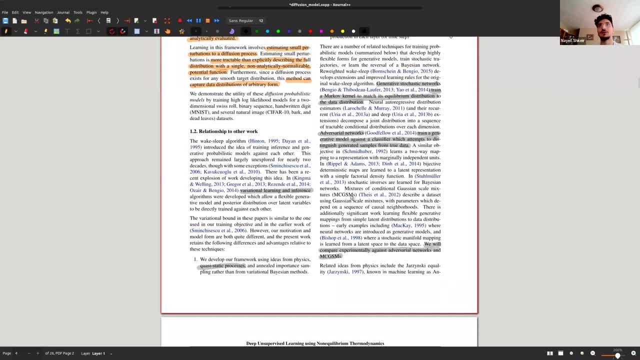 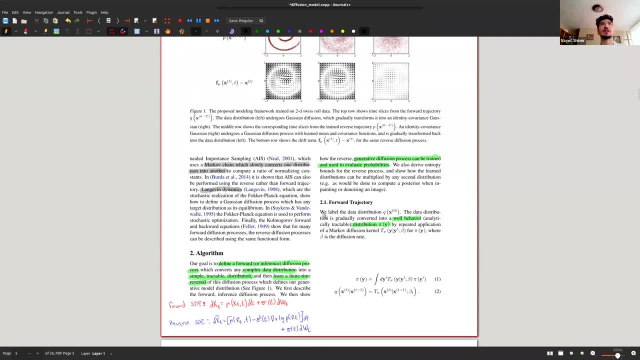 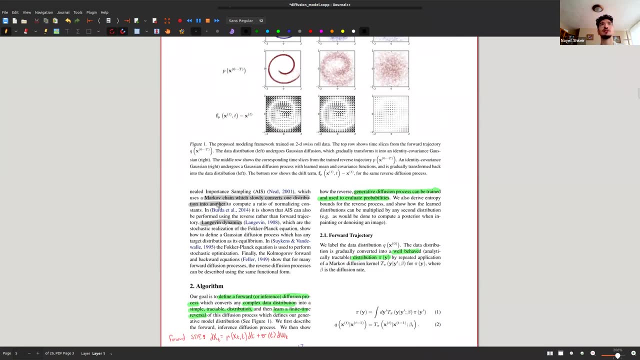 mixtures of conditional gaussians as well, which are sort of again sort of good generative models, uh, but anyway. so i think get get to the algorithm a little bit, okay, so this is another important part. so so they use something called annealed, annealed important sampling. so which is the mark of change? 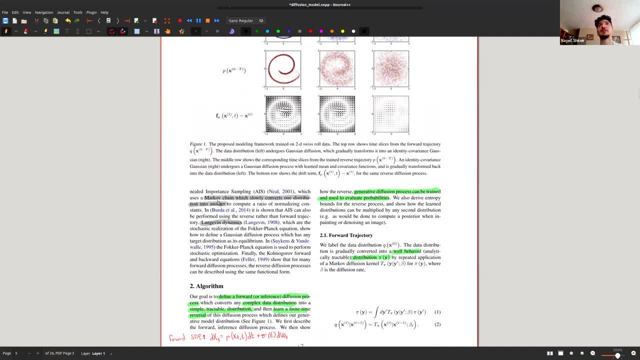 to convert one distribution to another. and so this is pretty important because you can't, sometimes you can't sort of use important sampling because, uh, the distribution that you sort of use to predict the distribution that you want to know about is can be just completely different and just useless. 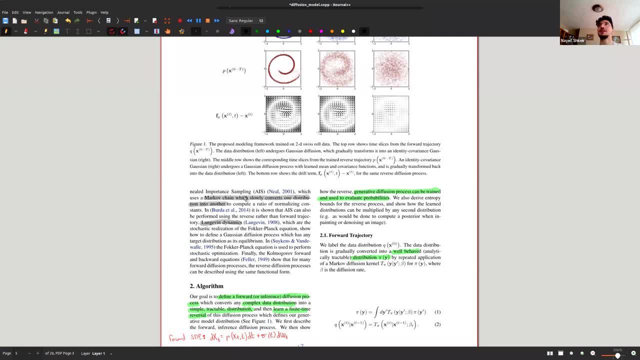 and so you sort of construct a mark of chain from one distribution to another and you sort of um go from move from one to the other in some sort of space and then use uh weightings, uh onto the sequence of the of the mark of change from one distribution to another. but i don't think it's. 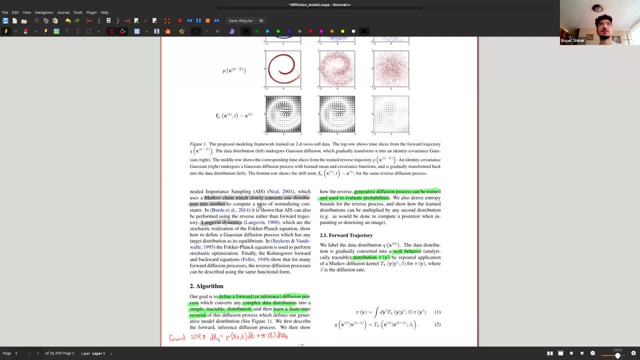 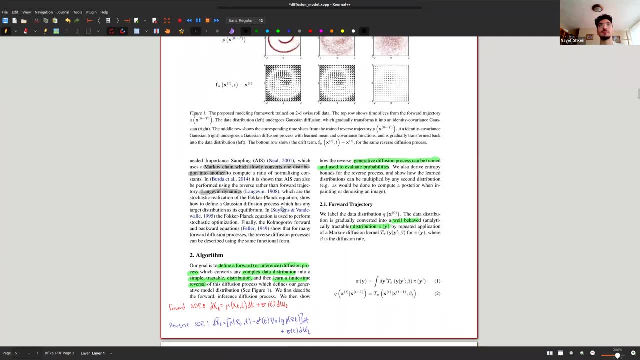 super important for this paper: um, it's just the use of ones, uh, and then so they have a launch one, dynamics, which is sort of. this is more sort of um, evolution of distributions, and so this is where this reverse property comes into play. so this is why this whole diffusion- 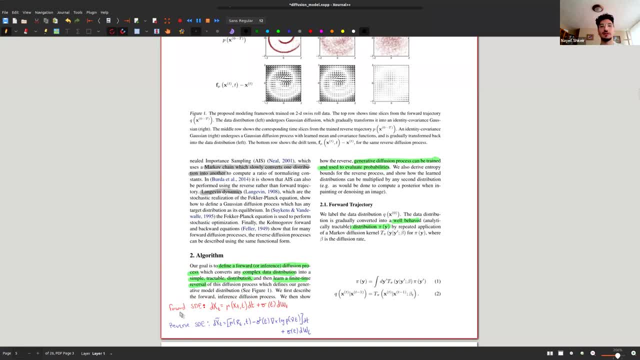 model can work is because you have some forward sde. so okay, so this is your, so this is the evolution of you. let's say, some variable x and this is your drift, so mu, which drifts you to some certain area. so it could be so if this is zero, so it will drift you to sort of mean zero and this is your. 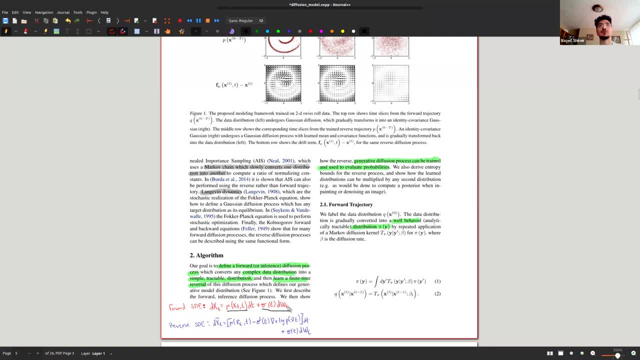 uh, the noise term all right. so this is your random gas noise and for this sde you can get an analytical form for a reverse sd. so in reverse time, so starting from a a point, so in this forward one you sort of move along some space from this point to the other and so you have a reverse sd which takes. 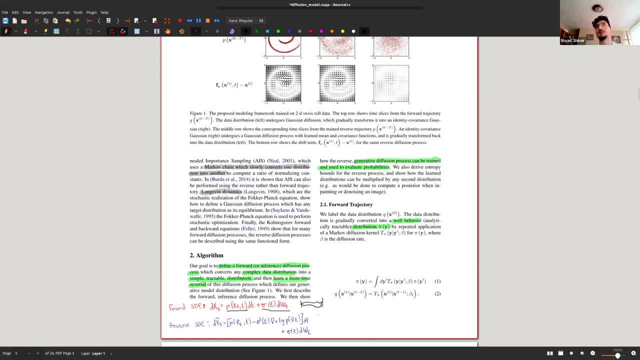 you from this point back again to the, to the initial condition that you started in the forward sd, for which is, i mean, it always blows my mind that you can sort of have reverse some stochastic process like this, but yeah, um, how do you reverse it? but when you look at the reverse process, you're 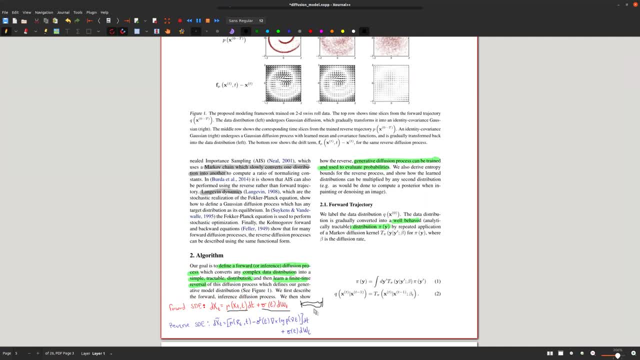 still at, uh, noise, right, the, the, oh. what is the dwc in that one dw? that's just browning motion, so that's just uh, you can imagine that as being a normal, exactly. but but again, in the second part you also add noise and you still reverse it. yeah, because, yeah, so there's still stochasticity in. 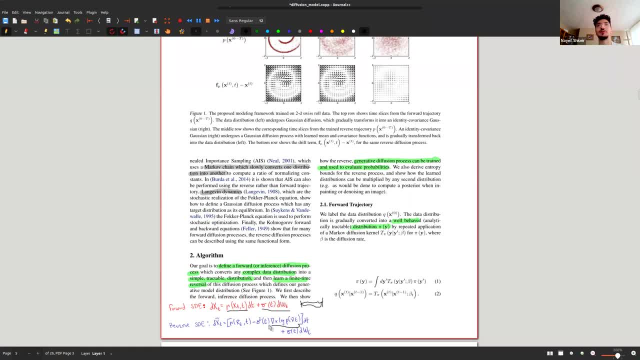 there. but you're going along sort of this gradient which is important here, which sort of drifts you in the right direction and because your, your, the, the sigma square, essentially sort of counterbalances the, the update harder, yeah, and then you add from the, from the additional, 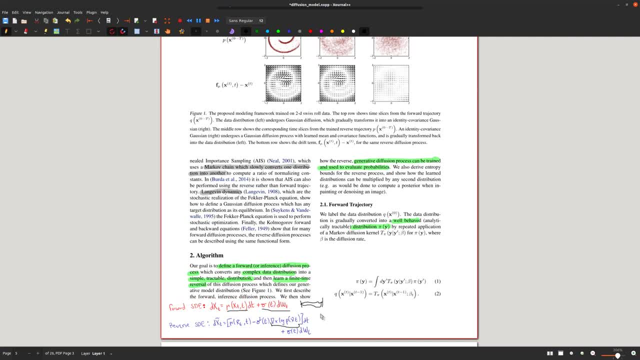 noise. so essentially, your, your gradient term wins over the noise term in the reverse, yeah. so this is, yeah super interesting. and there are other machine learning models which actually, um, use stochastic differential equations in their training and sort of exactly predict this gradient uh. so it's a pretty basic kind of uh method. that's a little bit harder to use, um, but of course 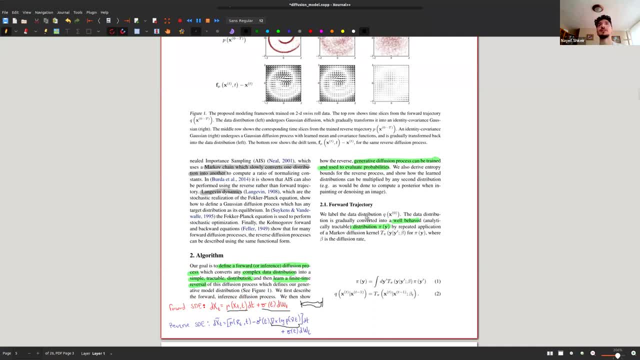 you can just use it in the right direction and you might have some problems. you might want to use maybe some more uh distillation to help you a lot with that. but yeah, this is something that i'm going to talk a little bit more about and i'll just get myself up in the Judaic. 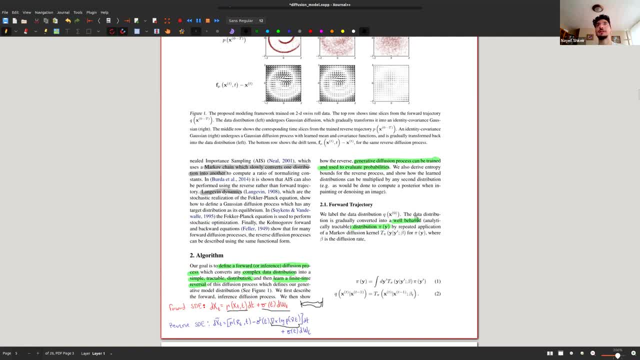 now and then i'll just tell you a little bit more about what i'm talking about here. but this is actually a very important thing in a lot of the uh delta. this is a long expression of the log of the distribution, but anyway, so that's. those are other methods, so they're slightly. 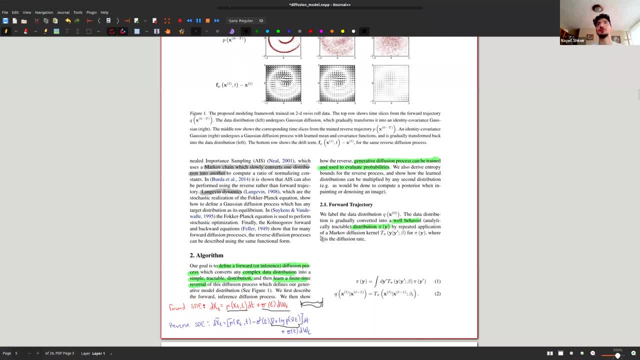 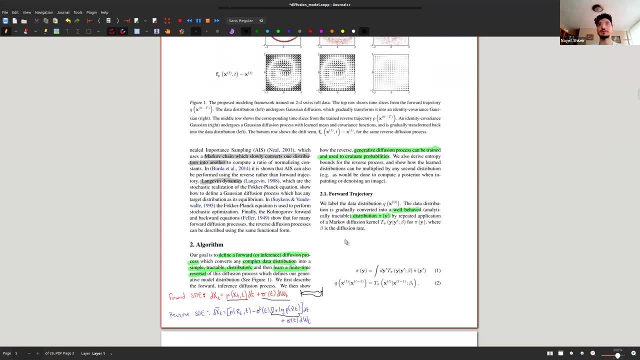 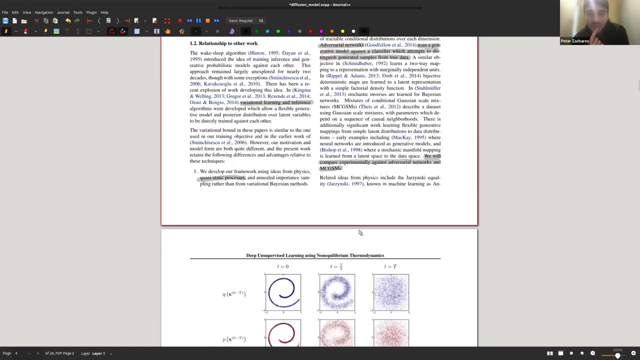 newer with the Markov diffusion kernel, where beta is the diffusion rate, And so this diffusion rate sort of varies along your Markov chain. Okay, so this is just your normal update. So this is literally- The diffusion rate is time invariant, isn't it? 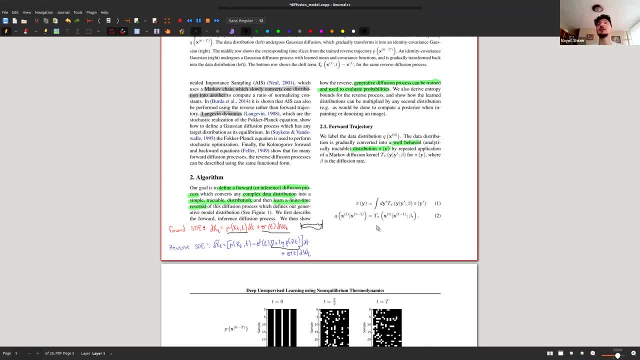 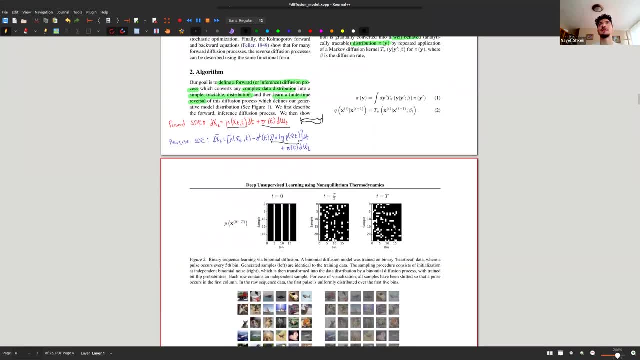 It's a constant or no Here? no, it's the expected T. Oh yeah, I see, I see yeah, And so they say later that this can be learned, or you can set it deterministically, depending on where you are in your chain. 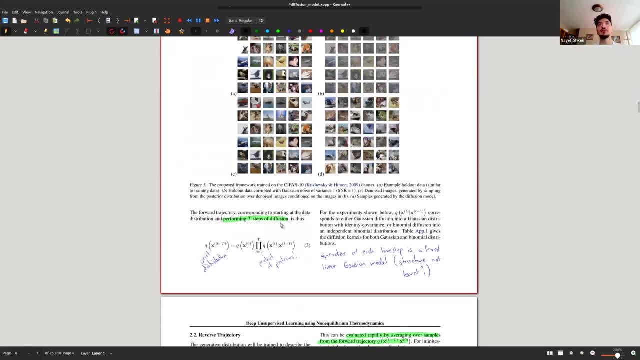 But yeah, so the forward genetic response is starting at the data distribution, performing T steps of diffusion, And so you have your joint distribution and it just becomes a product of your posteriors there. And so for the experiments it corresponds to either a Gaussian, 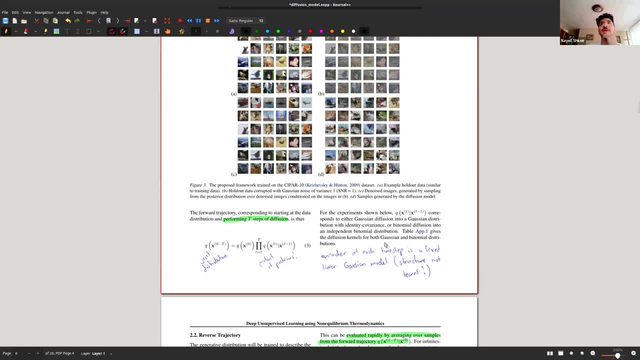 or a Gaussian distribution of identity covariance, because that's sort of the easiest to work with, And so the encoder at each time step is a fixed linear Gaussian model. So in a VAE you're sort of learning the weights of your encoder network. 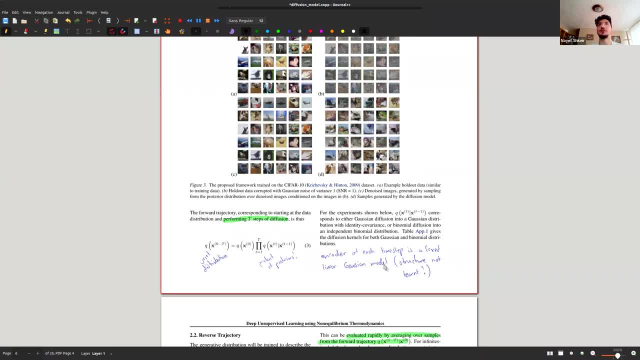 But here you're not learning any weights, You're just sort of learning your- Sort of it's fixed right. So at each time step you have a fixed model that you don't need to vary the parameters of the encoder. 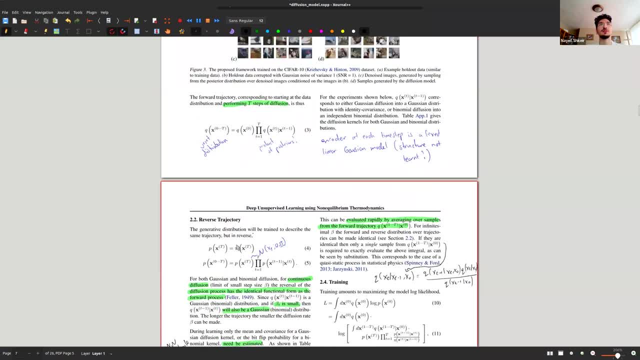 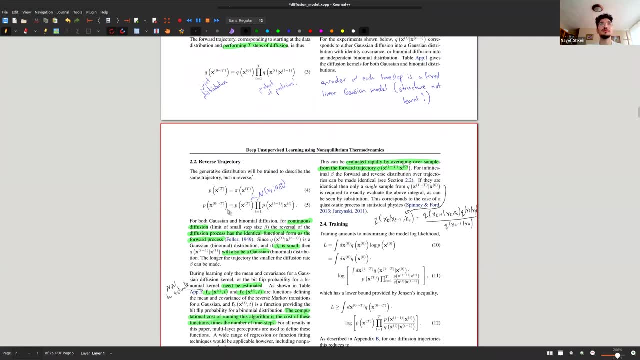 Okay, so this is the forward trajectory. and then there's sort of the reverse trajectory Where it says, okay, the genetic distribution will be trained to describe the same trajectory, but now in reverse. And so you start from your normal distributed isotropic Gaussian noise at X, capital T. 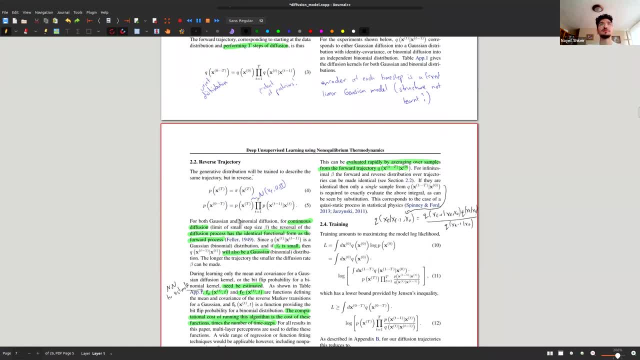 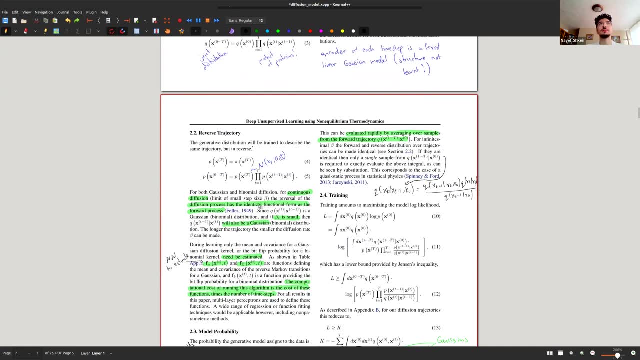 and then you go back to your data, X, zero And so okay, so for both the Gaussian and sort of the idea of binomial diffusion example, so the continuous diffusion limit, the reversal diffusion process, has identical functional form as the forward process. And this is what they mean by sort of this SDN right. And this is what they mean by sort of this SDN right. And this is what they mean by sort of this SDE problem here. And this is what they mean by sort of this SDE problem here. 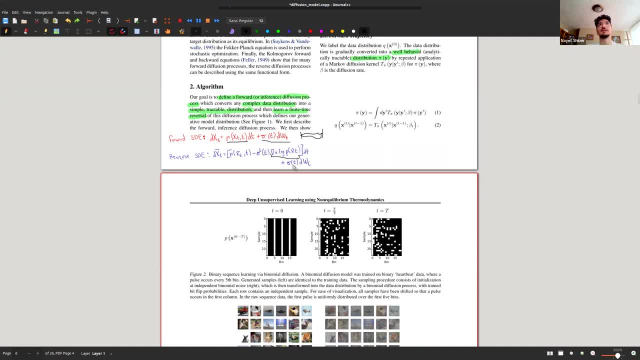 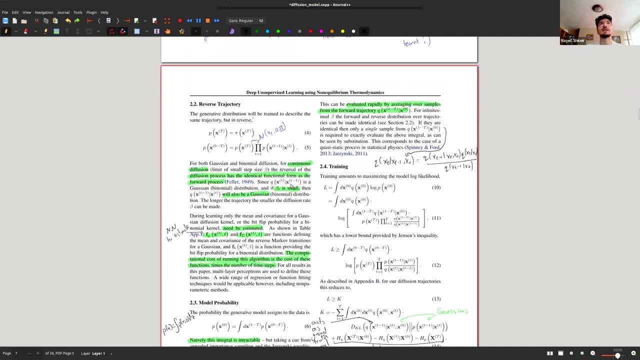 So it's very so identical function for me. You have your drift term and you have your sigma T. for your variance, You can write both down analytically And so, since this- So I have a quick question: The DDP that is in the reverse process. 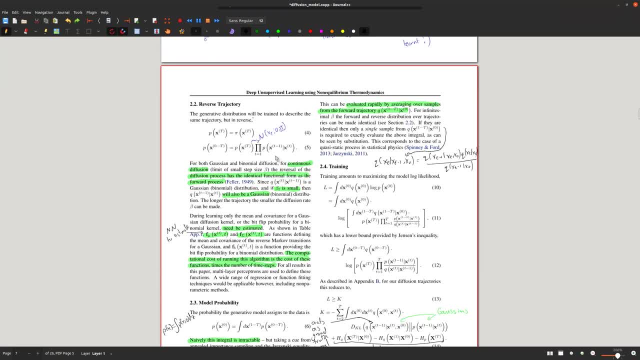 is that parameterized by something? Is it also data dependent or is it completely data independent? It's only dependent on the data from, like the previous Gaussian noise right. So it's, as in like, dependent from the previous step in the Markov chain. 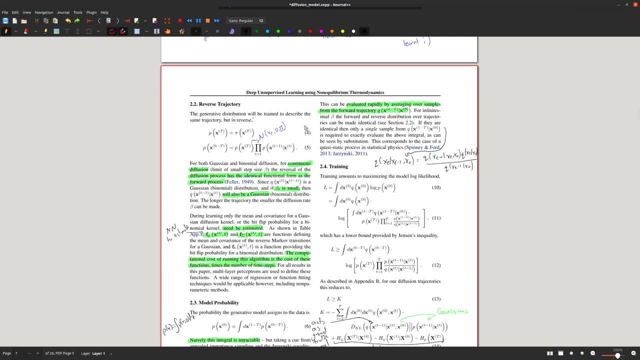 But the it's a product of P, of these transition elements, right? Yeah, I think that the mean. and the variance of the P, because it's a normal- Parameterized P, yeah, Is it takes, it's a. both of them are calculated. 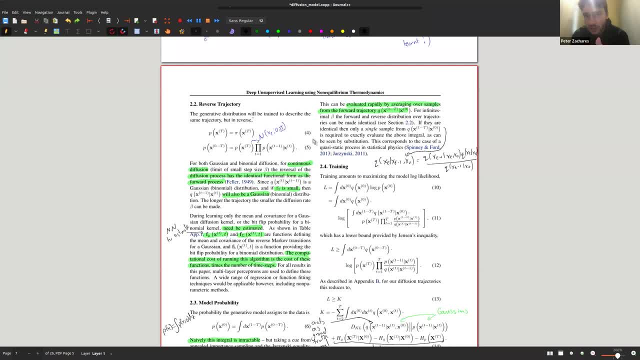 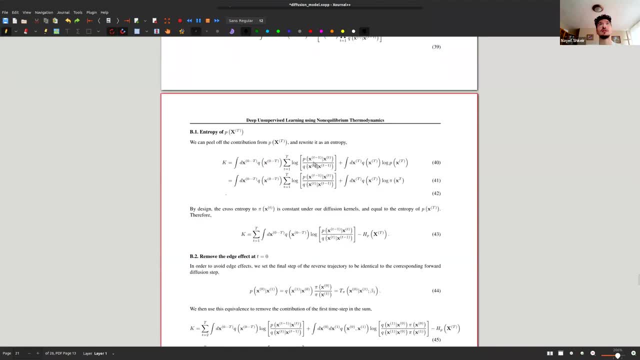 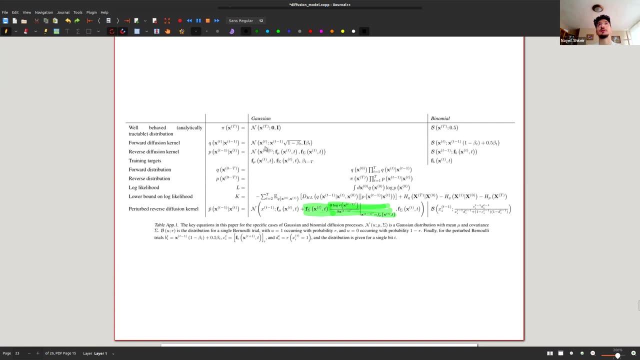 using a neural network which takes into account, you know, count, the like, the previous time, steps, representation. So they say it, they show it nicely at the end in the appendix. So here, so okay, So your P is gonna be some mu and sigma. 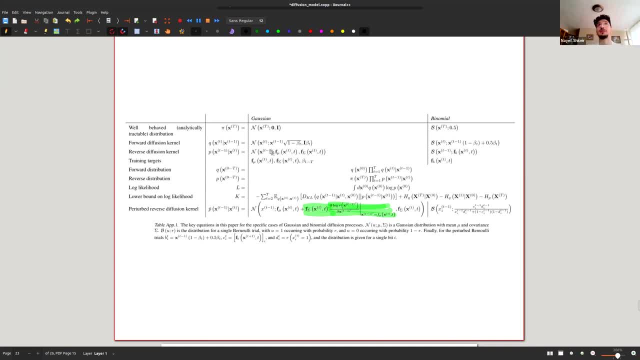 that you calculate from your neural network and you update the previous. so you update T with those weights to give you X T minus one, And so it yeah. so it doesn't know about any other outcomes. It's really just that- Yes, complete Markov. yeah. 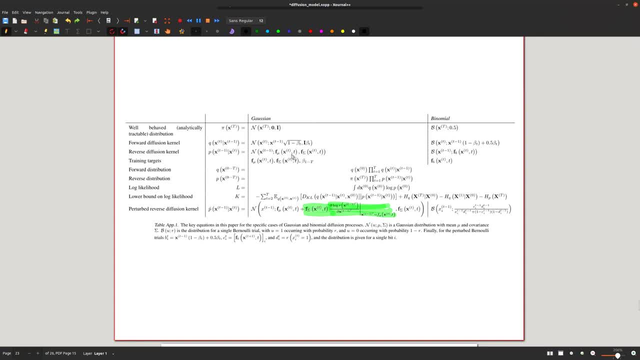 So we know that at the very, very, very first reverse step we have guaranteed Gaussian input right, So there's nothing that can distinguish two different images. Yeah, And yet somehow, on that very first step, it, it can create. 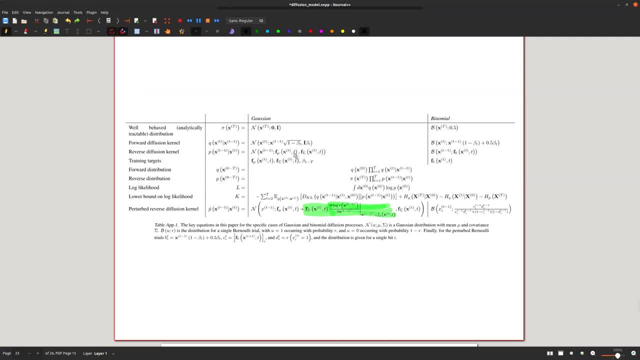 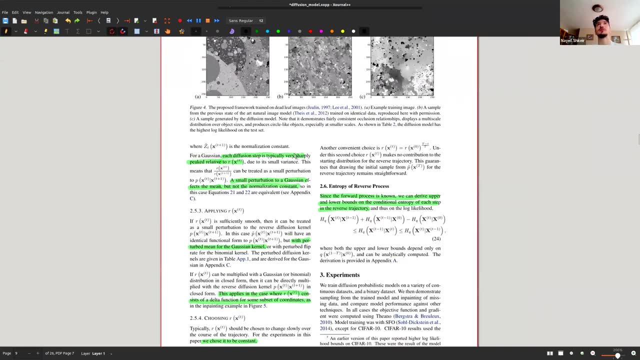 it's something in there that is. that is, that it makes it makes it slightly more differentiable, right, Yeah, it's because what you assume? well, you want the forward and the reverse process to be as similar as possible. 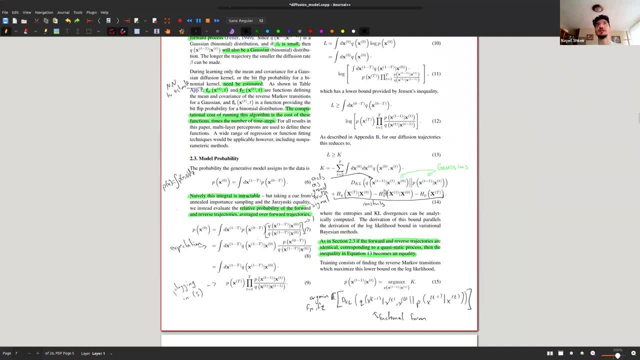 And so you train by sort of reducing this, the KL divergence between the two, the reverse and then the reverse process, And so because in the limit they're exactly the same, And so this is why, yeah, you're saying yeah. 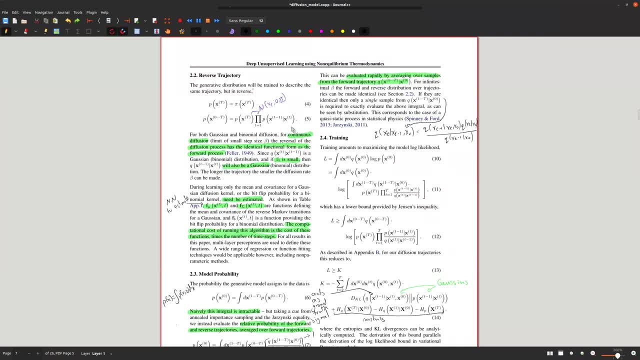 you're sort of able to to go back in time, But I still don't really understand how, how, how, how the same distribution can, can can lead to in, in, in, just the very first reverse, reversal step can lead to something that is not. 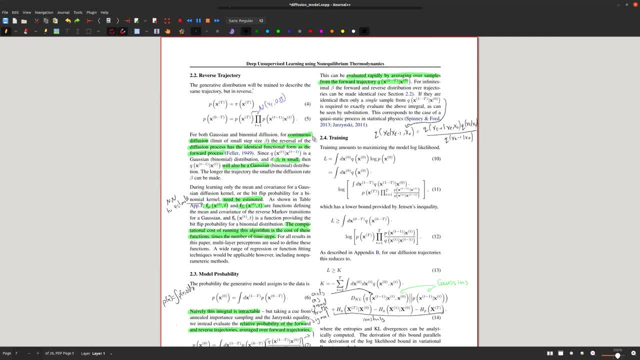 not isotropic Gaussian, Because, because somehow you must have this, this, this symmetry, breaking where, where, where two different inputs must at some point, you know, create- and this is still some- some, some slight leftover at the very end state. 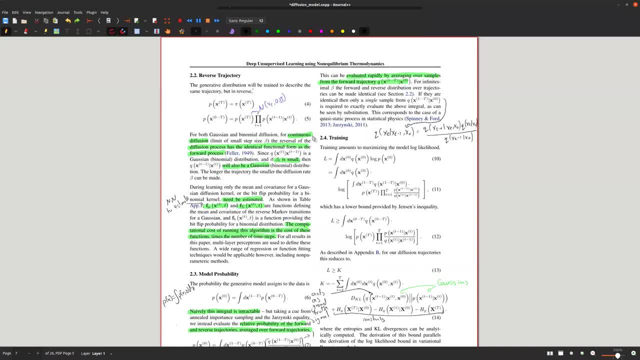 So so it's not really isotropic, but rather there's still some small Well in the limit. it is going to be completely isotropic, but I guess it depends how large you pick your capital. T is Yeah, But even if it is completely isotropic, 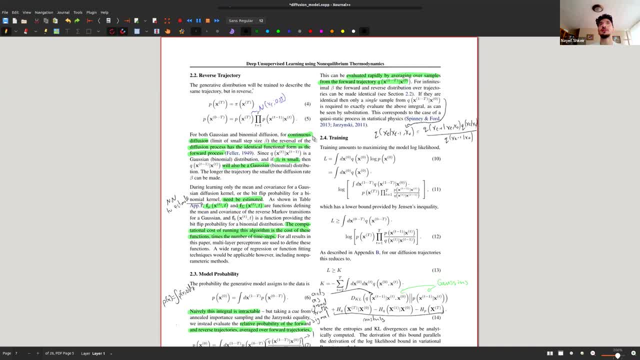 you are, you are still able to sort of go back in time because you sort of you do learn your mu and your sigma for the reverse transition. Arvid, I was, I was thinking about this. I mean you know I was thinking about this, I mean you know. 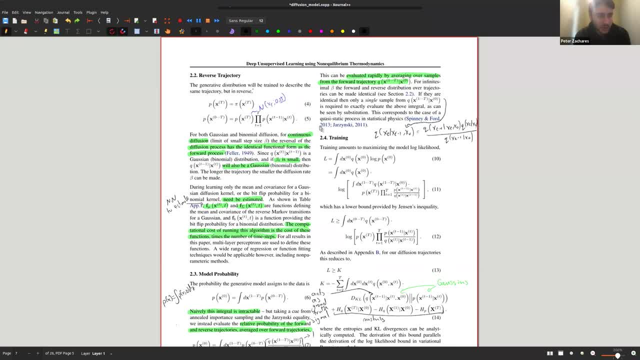 maybe this is a simplistic way of looking at it. Well, it probably is. It's just there's some locality here. So if you get a sample from like the upper quadrant of a mean centered isotropic Gaussian, it would map to a different set of images. 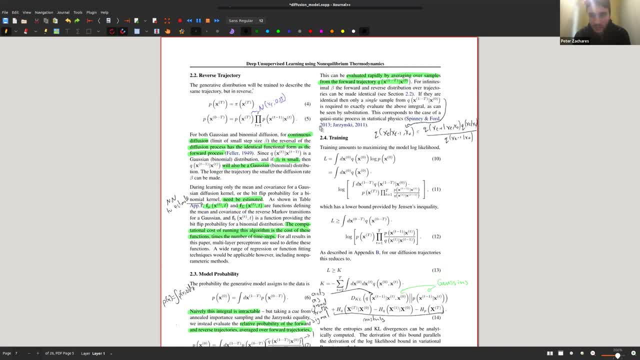 in the input space. Is that the-? But it's not the encoding. that is because the encoding keeps the same dimensionality as the input picture, right? Yeah, So you would expect after many, many steps that the whole picture is essentially noise, right? 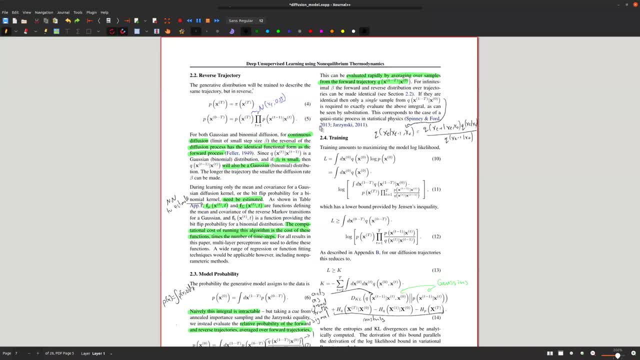 So so two pictures that look very different on the left-hand side. they look identical on the right-hand side, right. And because the machine only takes its input the very last image in the very first step. it must mean by symmetry, that the step before 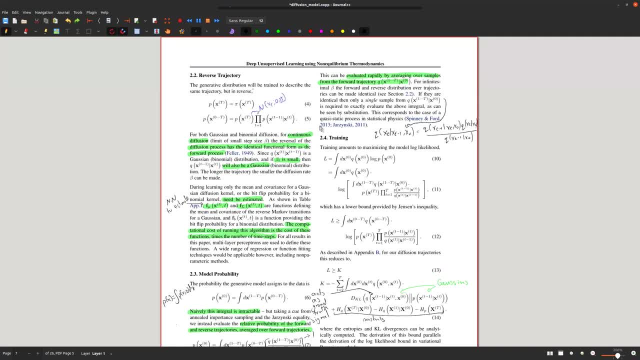 that must also be completely isotropic. Otherwise, Because it makes use of isotropic redistributed input. Do you mean in the forward process or the reverse? In the reverse, Because if it's only a Gaussian right, If it's a Gaussian evolution, 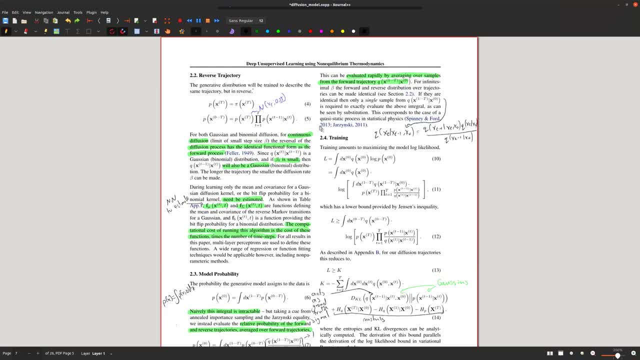 again, process or data processing. inequality means that you know you can't get information out of nothing And because the neural network, if I can do that, you know you can't get information out of nothing. I understand correctly that the mu is a function? 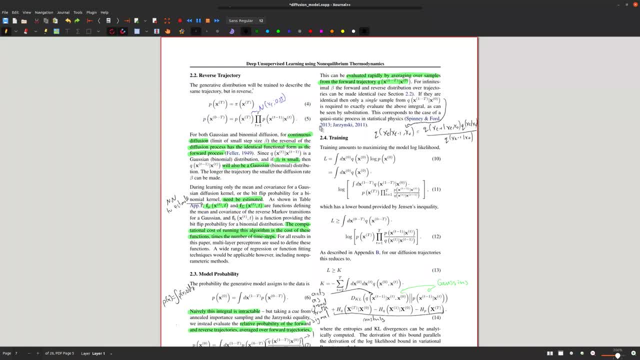 of the input data, which is again fully isotropic. At some point you would say that if all the input is isotropic, then of course the very first step is also isotropic, Then it's from the second step as well. 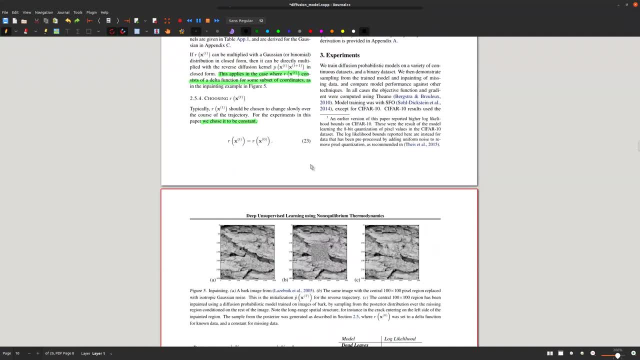 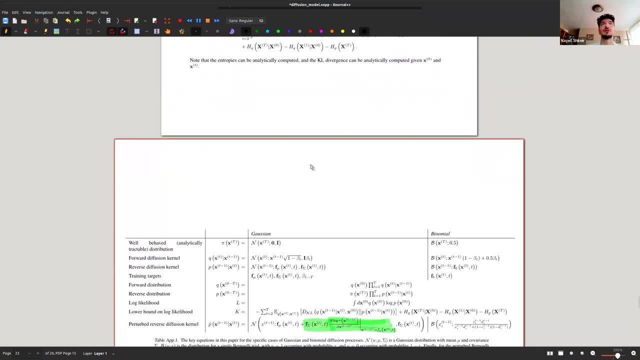 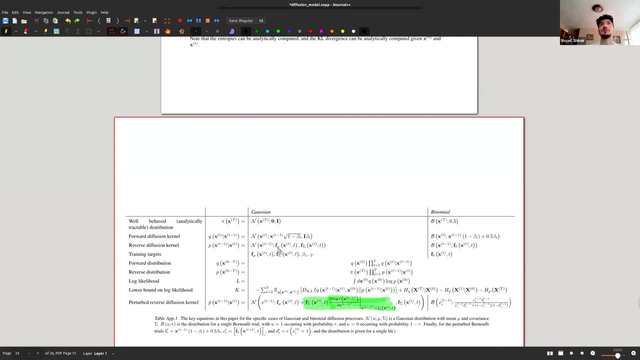 because it's all gaussians from there on. So I still fail to see where Mute is not gonna be from. okay so, Okay so in this part here. okay so, this mu is just, it is gonna be. 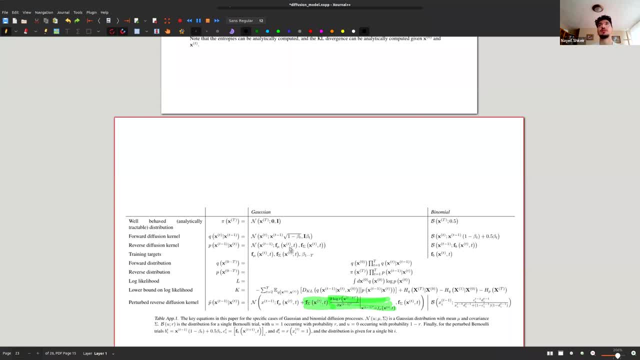 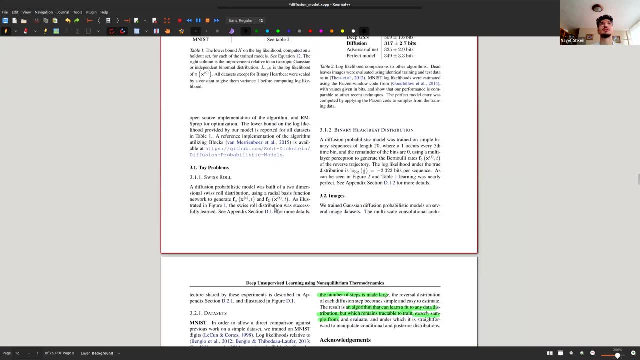 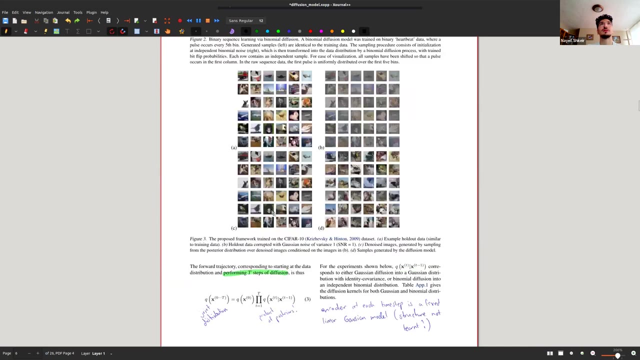 so it takes as input sort of your completely isotropic Gaussian, but Oh, also by the way. okay, I think this should answer If I go up. What is it? So the first step in the reverse process is here, right, 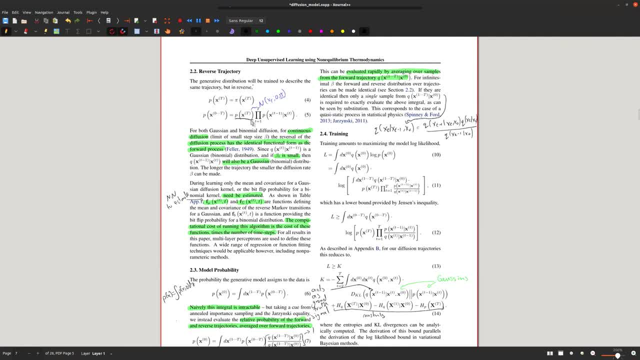 So this is your completely isotropic Gaussian. And then you take your next step and you put sort of your isotropic Gaussian in, But then you have your mu and sigma that you've learned from sort of minimizing the difference in distributions between the reverse and forward process. 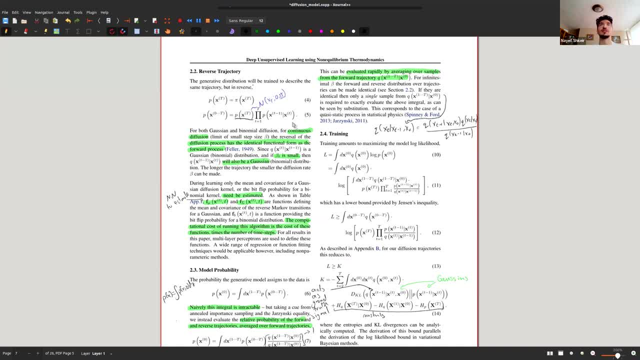 So it doesn't really matter that much that it's sort of isotropic Gaussian, right, Because you've learned your parameters, But the parameters are the same for all the inputs, right? So your No, what do you mean? the same for all the inputs. 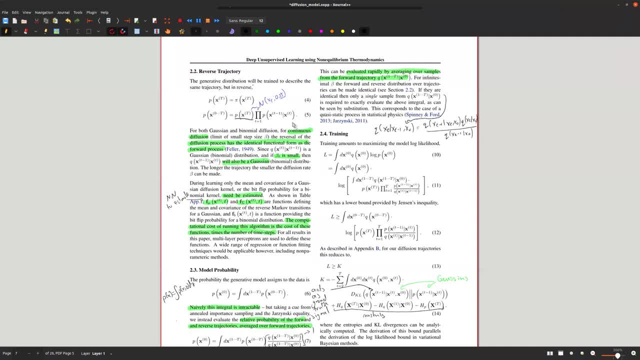 Well, the functional form for the very last step is the same for all inputs, right? Because the function only acts on X of capital T, But mu and sigma are different for in different positions in the Markov chain. Yes, that's, I agree. 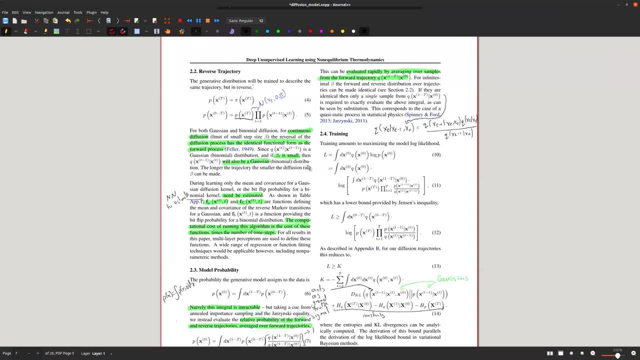 But again, if the inputs are isotropic, the outputs also must be Maybe not isotropic, but indistinguishable, right? So two inputs, say two inputs at X zero that are different lead to the same X capital, T right. 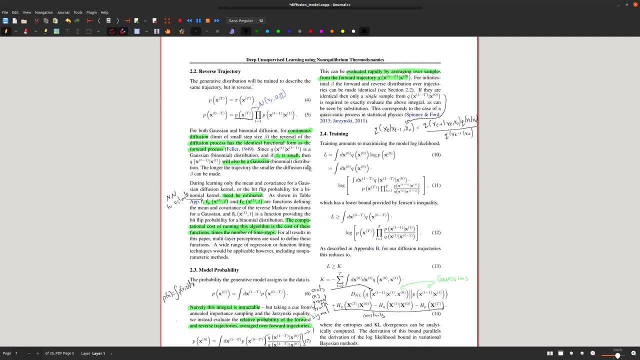 So we have some kind of loss there. If you go X capital T to X capital T minus one, if it's a Gaussian process, it only takes X capital T as input. Yeah, Yeah, Exactly. So how can X capital T minus one? 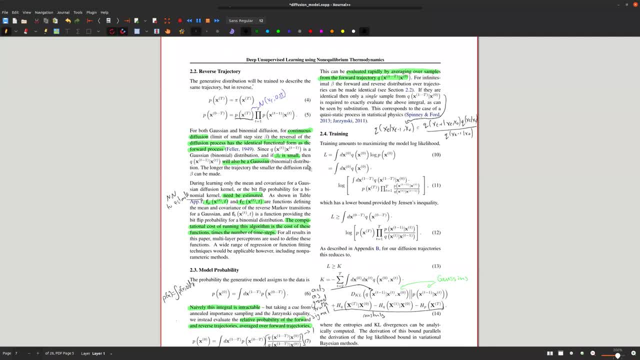 be possibly any different between the inputs, Because you modify it. You modify your X capital T to be a slightly less isotropic Gaussian right, Because with your mean invariant, so you keep modifying your X capital T, Oh, but the mean invariants. 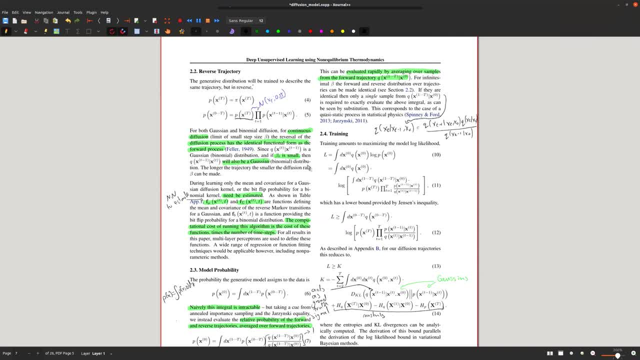 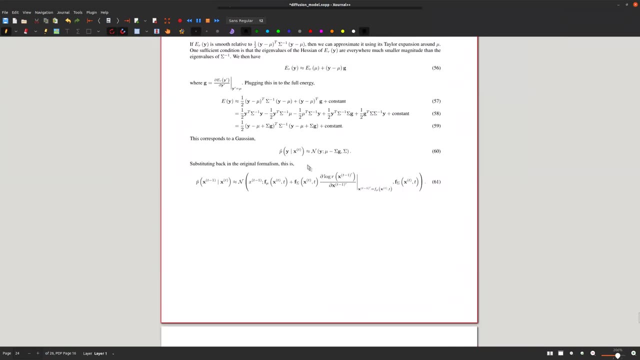 must be the same for both right, Because it's only a function of the last step, which is isotropic. But that's the drift. depends on the pixel right, Is that correct? The mu Depends on the pixel right, So you got different drift for different pixels. 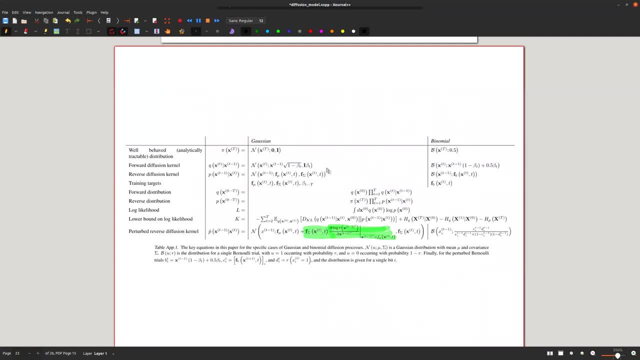 So maybe that could be. But that would only work if the very last step was not isotropic. There's still some residual information about the image left in xt. then you could see how it gets essentially rebuilt, each step a little bit and possibly cleaned up. But if it's truly isotropic, 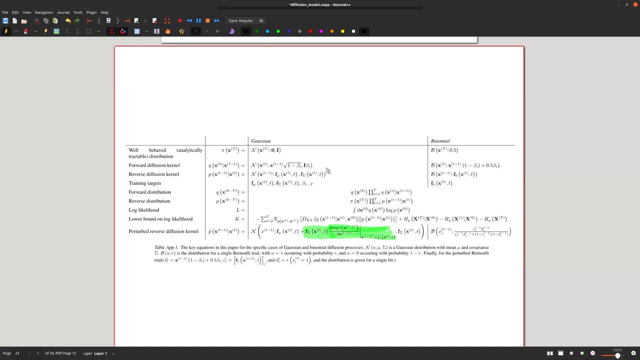 I don't think symmetry would sort of break that. Could it be that? Well, the reason- Maybe it works- because the isotropic Gaussian is in this case, when we're talking about images- is like A projection of the original distribution. Maybe projection is the wrong word. Anyway, 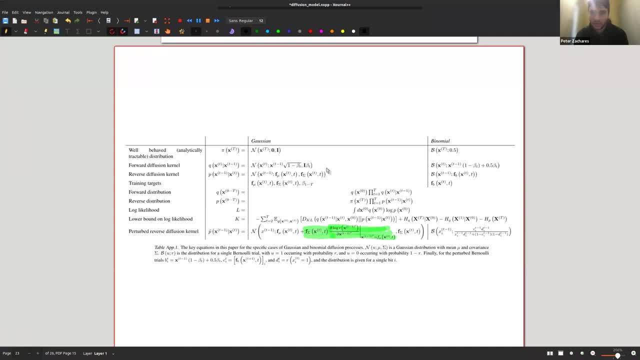 it's a distribution over image space And I don't think that the output of the model at the end of the diffusion process is a set of parameters for the distribution. The output is an actual sample, So you can correct me. So, for example, an image will be projected into the same dimensional. 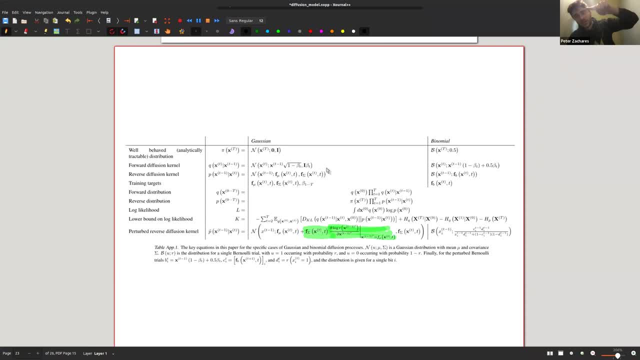 space. but if you plot all of the images in the data set, they should create an isotropic Gaussian distribution once they've been propagated through the diffusion process. But that means that each point in the isotropic Gaussian is actually an image. It's not like a pixel or something along. 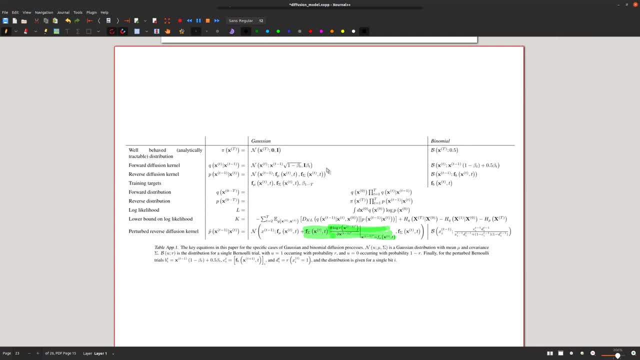 those lines. So you say that X capital, T is as a whole is like on some multidimensional Gaussian, But at the same time we know from the pictures that each individual one is also very, very noisy. But so then, essentially, we're saying: 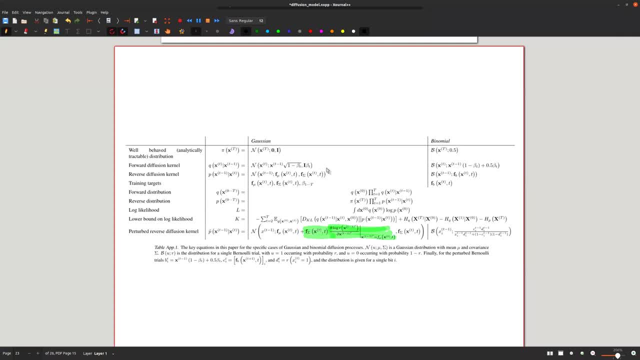 that each point, each input gets mapped to a different point at a very high dimensional Gaussian, Or I would say probably a different region, A region, yeah, Because that would make sense then. right In that sense, that then different regions of that. 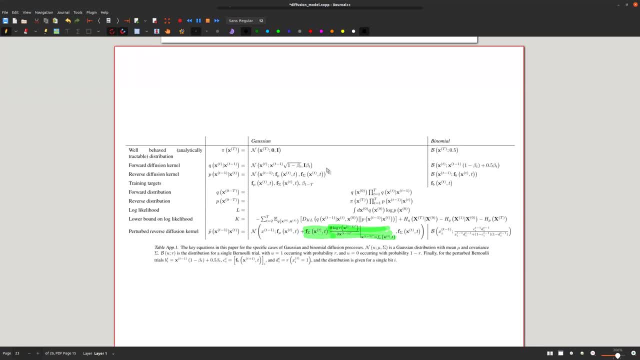 high dimensional Gaussian could then definitely map to different places in the original picture. I don't see how it's weird to have taken isotropic Gaussian as input and varied based on some mean and variance and to move it away from being an isotropic Gaussian. 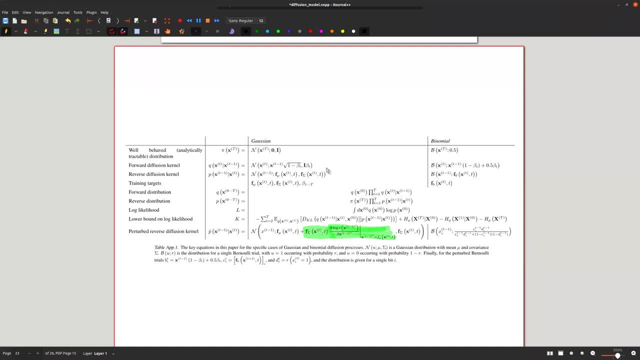 It's moving it away from essentially creating a difference between images, right, So that apparently the two isotropic Gaussians mean something different for the different input images. Where does the difference come from? The point is that you don't have a separate isotropic. 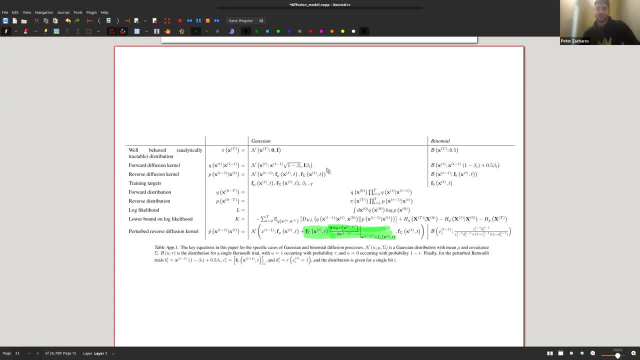 Gaussian for each image. The distribution is over the data set space, not the pixel space, Because it feels like when we add the noise, that we essentially do create the isotropic Gaussian on the image level. But you're saying that is not strictly true. We actually do it. Well, that's my interpretation And I didn't. 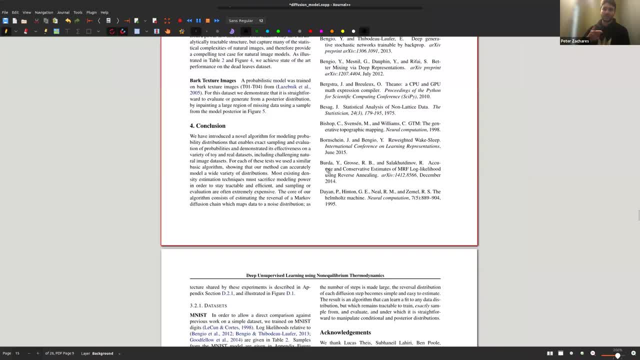 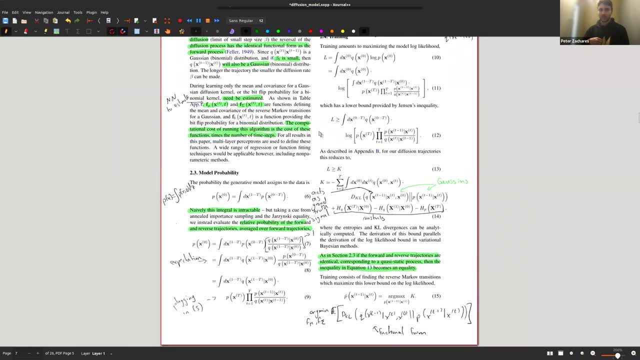 write this paper, But in the backward pass also, you're sampling from the isotropic Gaussian And then you're doing this reverse diffusion process. So in both cases you're not modifying a distribution. Yeah, You're modifying sampling, You're modifying samples from a distribution. 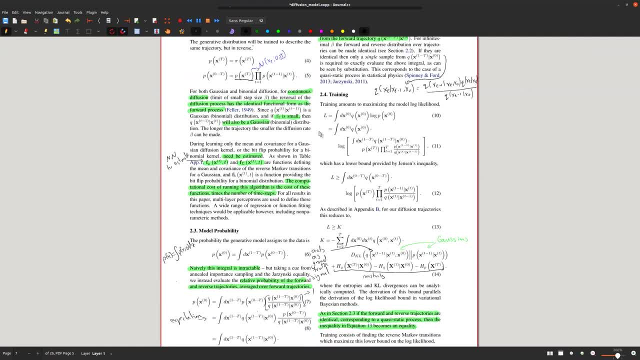 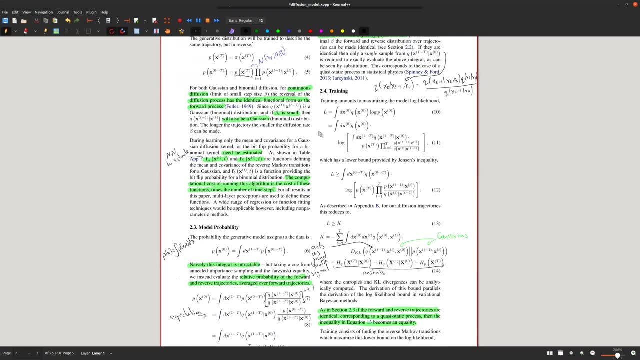 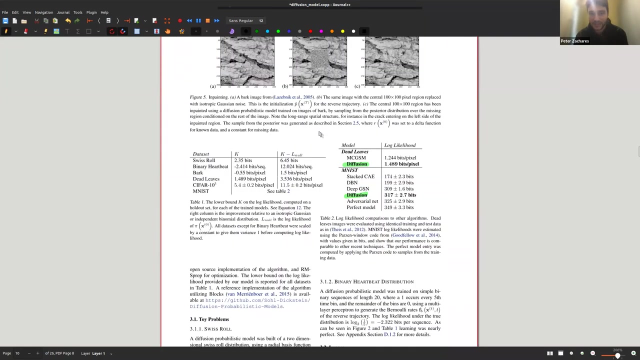 So when I give, say, these diffusion models an input to generate me an image, what actually would happen is: would I restrict myself to some region in that multidimensional Gaussian on the right-hand side? So, based on the CIFAR-10 generated images, I think that are there, that there is a lot of blending. 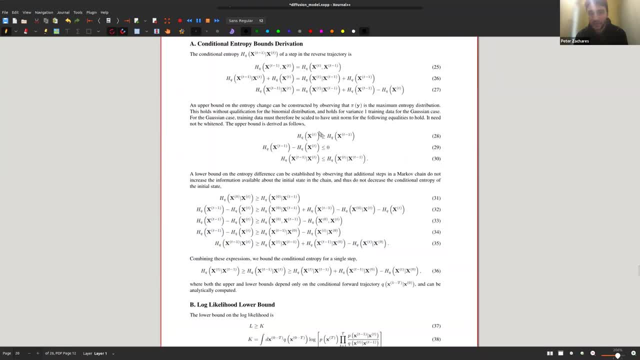 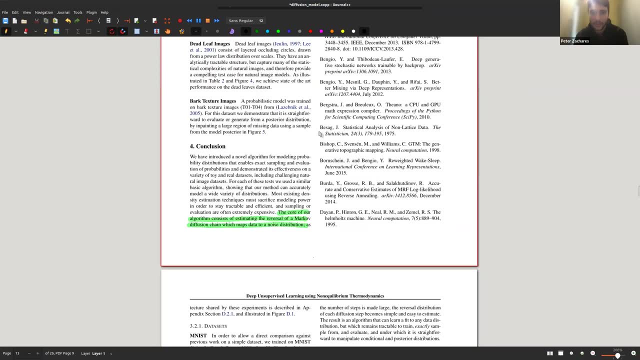 And so, yeah, I don't think a part of this paper that they didn't really do was that they're not here, They're up there, They're in the main part of the paper. Like, I don't think they know which region corresponds to which class. 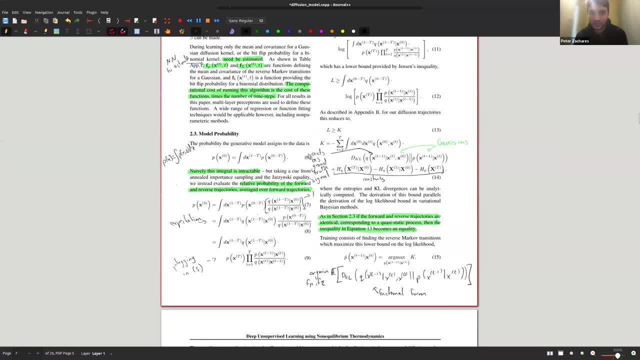 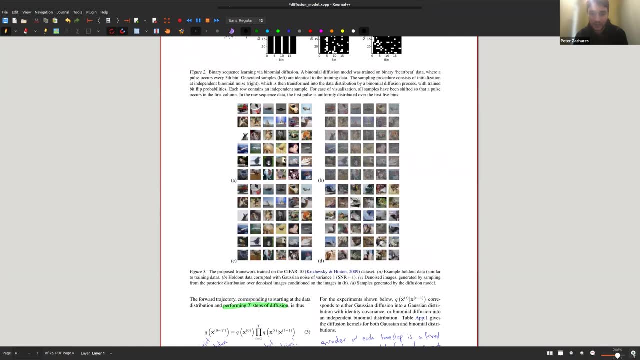 Like if you look at the images, they look so blind to keep going up Other than OK, there's C is just generated images where they sampled and generated, And if you zoom in on them so you can actually see them, they are such blend. 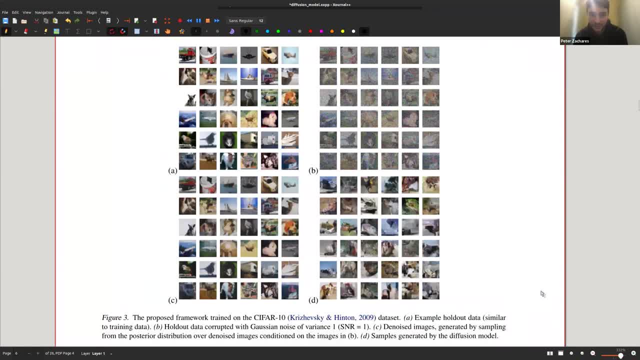 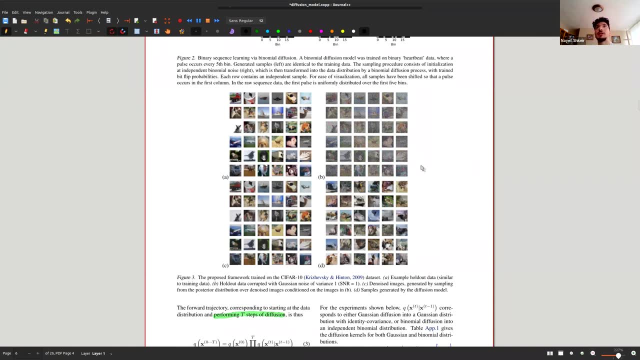 Like there's definitely structure that it's picking up on But it's not able to add the structure together to make a realistic image. But you're still starting from a complete well as close to an isotropic Gaussian for an image in 2D space as you can. 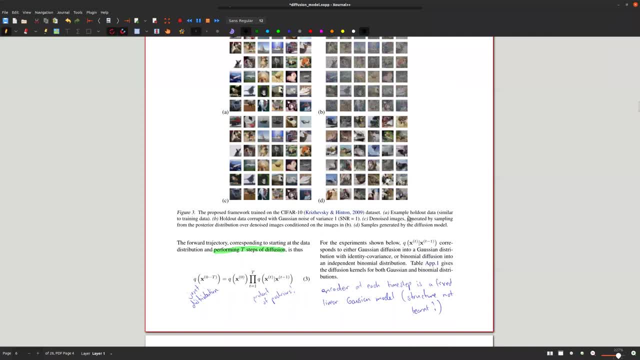 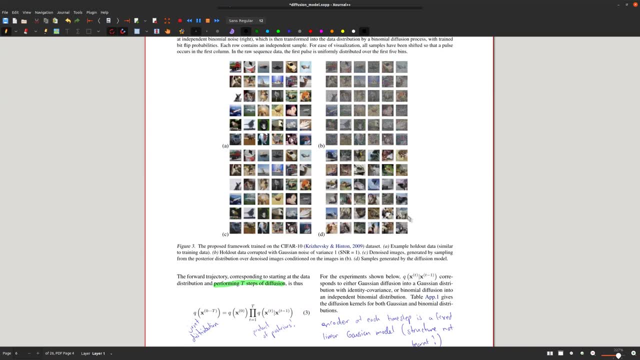 So would it be fair to say that the two images that are far away in the input space would also be in that Gaussian encoding space still very far away, that the noise that is added can't realistically put them close together because of this very slow, adiabatic updating? 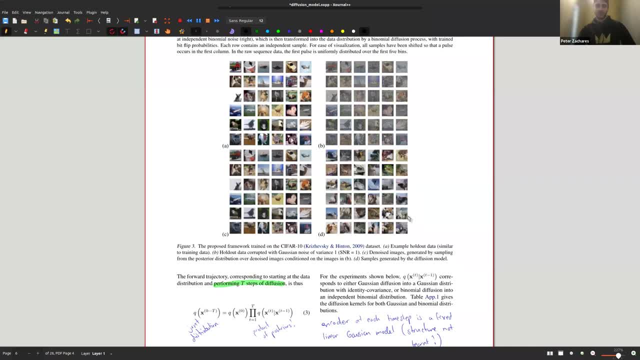 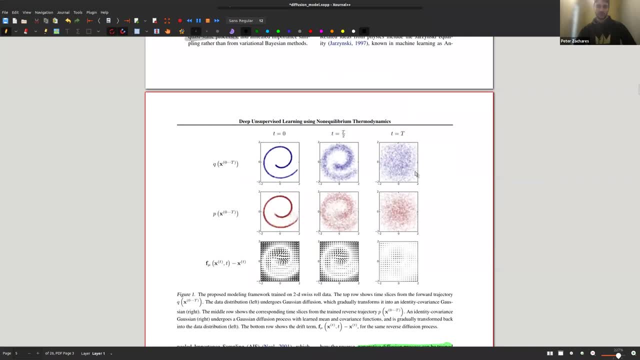 I would say so And I use the Swiss roll example that they have above. You can see that only points that are close to each other in both distributions. If you look at the third row, you can see the vectors that are mapped, like the diffusion process. 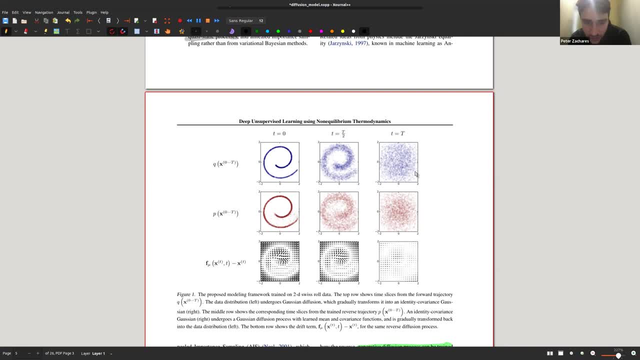 And so it doesn't seem like points that are very far away, Like any point can be mapped to any point, from the isotropic Gaussian to the Swiss roll. Sure, sure? No, what I mean is say, take the Swiss roll example. 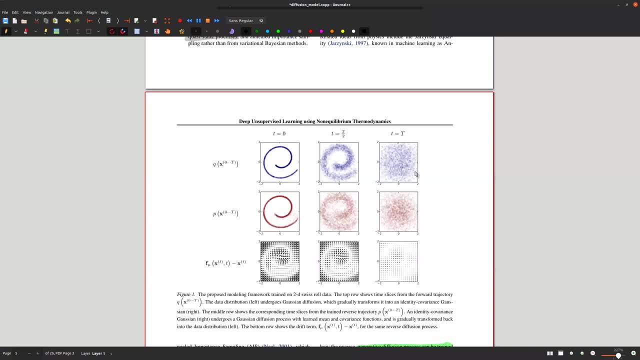 Take the first picture and rotate it by 90 degrees. So now we have a different input picture. If I run it through the diffusion process to the right, I still get a cloud that looks very similar than the than the cloud produced by the initial image right. 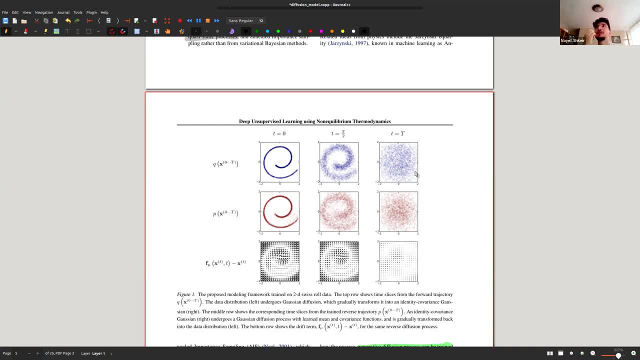 But so here, maybe here- the Swiss roll is not an image. It's like a two-dimensional space that you're projecting onto another two-dimensional space. So the data points here are not like that. That's why, if you rotated the Swiss roll, you'd have to train a new model. 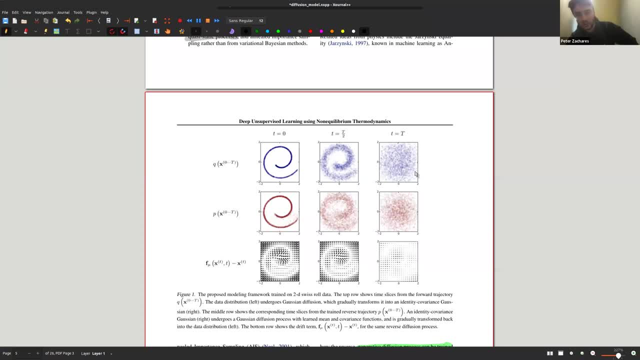 because it's a different distribution now, Whereas when you're doing it on the image, like a data set of images, your data, you're doing it over the data space, not the image space like of each image. I think I see what you mean. 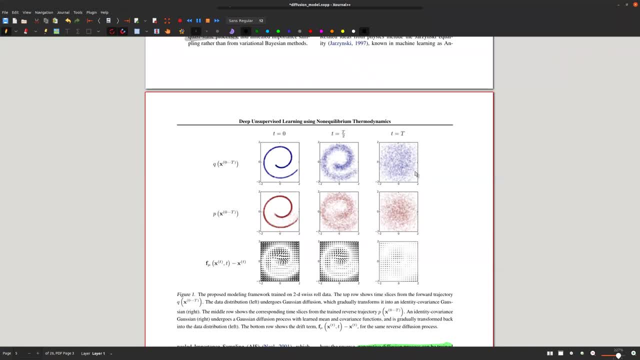 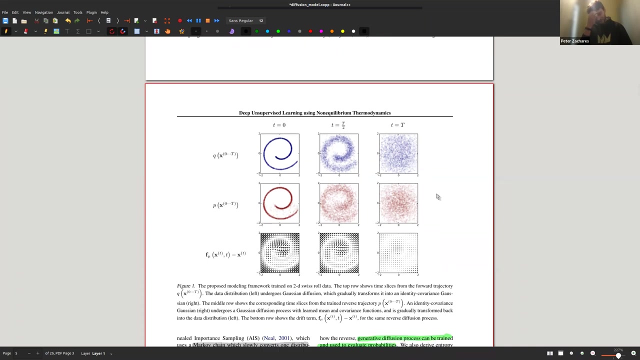 So each dot in the Swiss roll is not an image pixel but a representation of an image itself. That would make sense, Miguel, because then, but their pictures seem to imply it otherwise, right, Yeah, I agree that, like from this thing, you could think like: 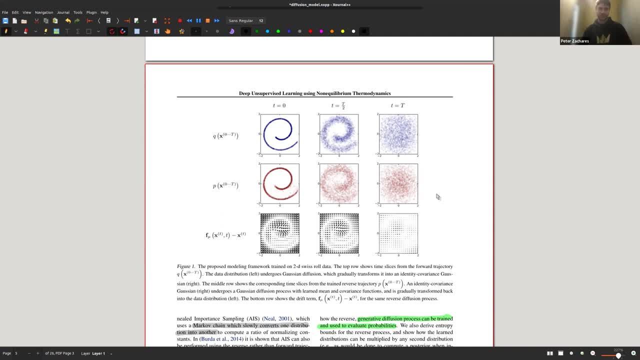 oh, why don't you just switch the rotated 90 degrees? and how can it express both Yeah, because then, yeah, that makes sense if all we say is that the encodings themselves over the total ensemble are Gaussian. But that is, yeah, what the normal encoders does as well. right? 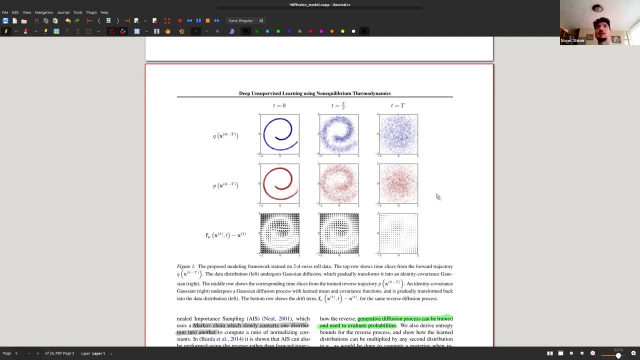 Or variation encoder at least. Yeah, but I guess in this case I mean it's fully defined by normal Gaussian. You don't have any sort of parameters that you're learning in a neural network. Yeah, Yeah, Okay, So okay. 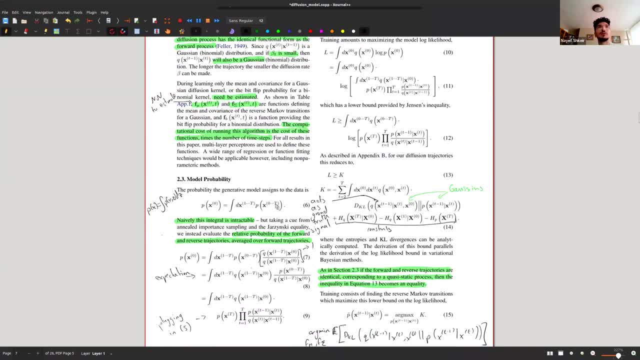 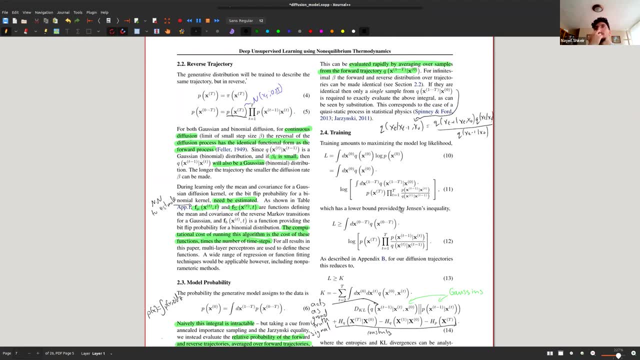 So that's just the learning And so you have yours. only have like 15 minutes, but so I'll get to the loss function. The loss function is really similar to the evidence lower bound for the variation autoencoder. So the main part is: 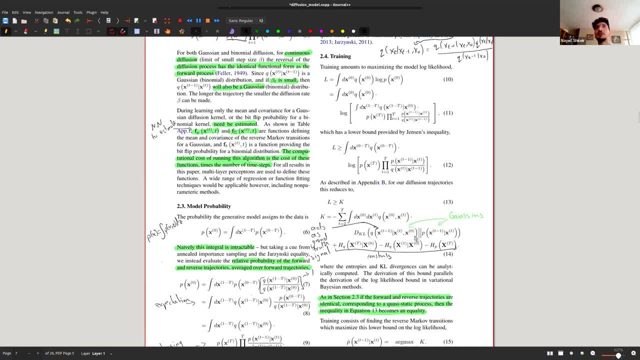 is this sort of KL divergence between two Gaussians. So you have your ground truth signal which is going to be your image, that you've sort of an image in your forward Markov chain which is going to be a ground truth, And then you sort of calculate the KL divergence between that and the image that you're sort of. 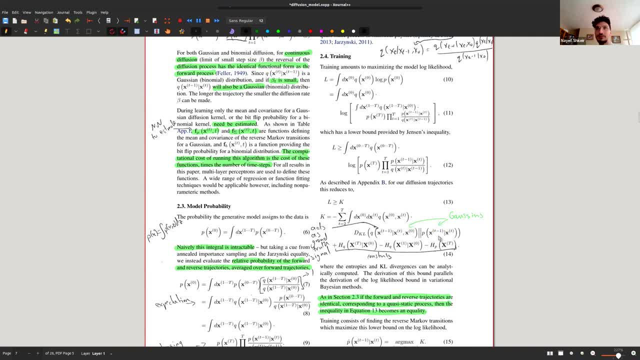 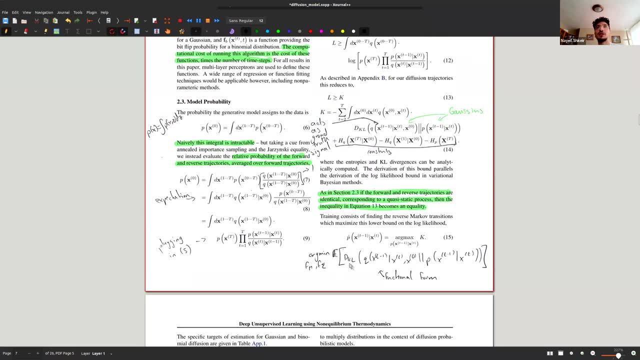 generating from your, from your isotropic option. Okay, And so, yeah, so they. so you're trying to minimize the scale divergence based on some mu and sigma. And this scale diverges between because it's the KL divergence between two Gaussians, so it has a functional form. 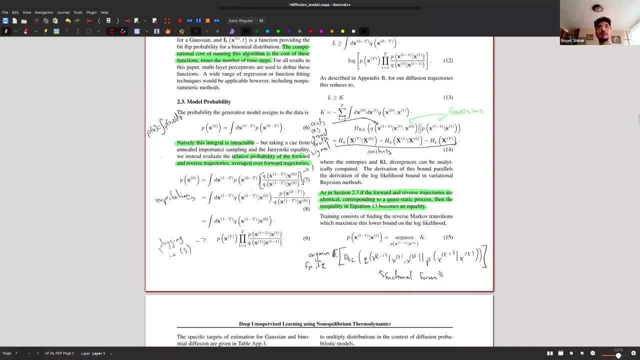 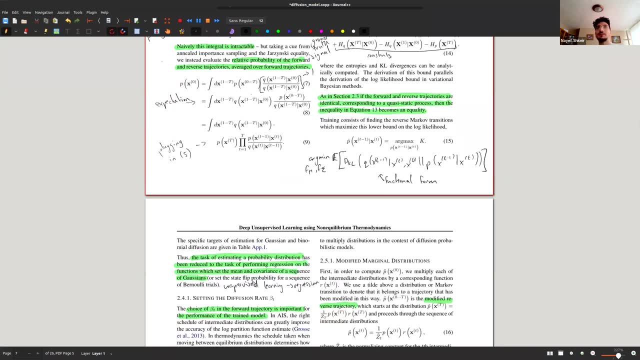 It has sort of a nice analytical- you can write this analytically. And so then they say so. they turn an unsupervised learning problem, a regression problem, into a regression problem where you only need to learn a mu and a sigma. 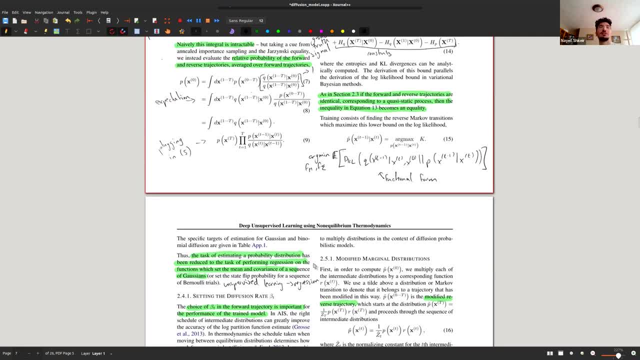 Which I feel like makes this problem sort of really really nice. You go into this sort of, I think, like a complicated, unsupervised learning problem and then you just you transform it into regression, But okay. and so then there's, they talk about sort of setting the diffusion rate. 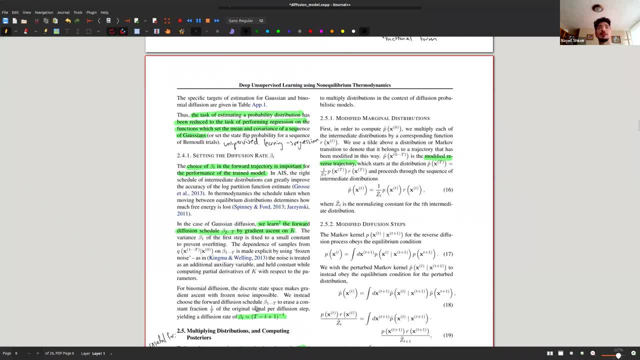 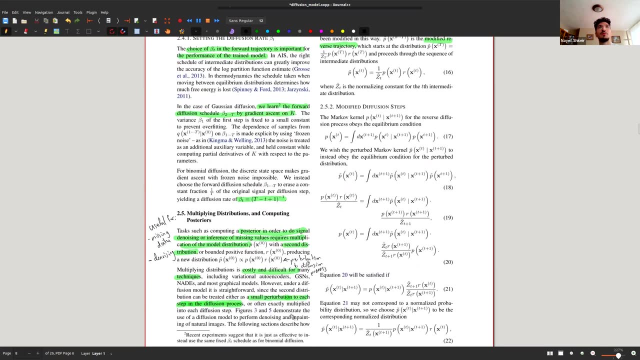 so you can learn the diffusion rate or you can sort of set it yourself. So they found out that even if you learn the diffusion rate or if you set it with this one over a capital T minus C plus one, it doesn't really change anything. And then they go into how this is useful for missing data or 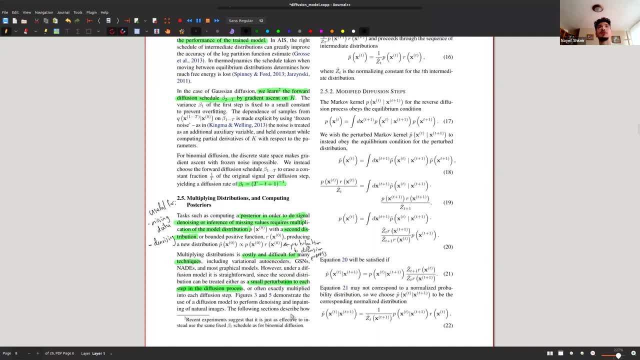 denoising data, And so they do this by perturbing the diffusion process, And so okay. so so computing a posterior, in order to signal denoising inference of missing values, requires multiplications of some model distribution. for the second distribution, which they call r, And this multiplication will produce a new distribution, p, tilde. 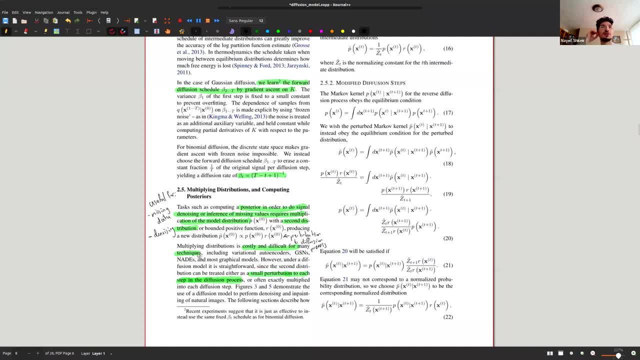 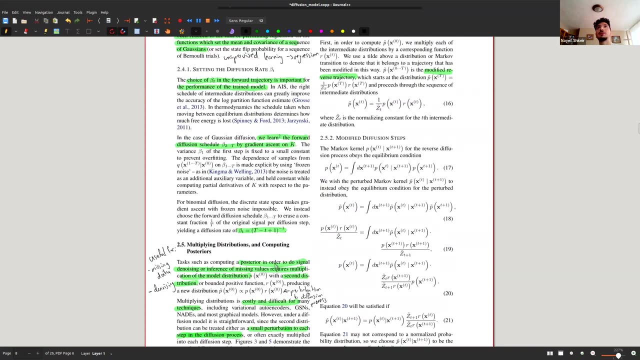 And so, yeah, so multiplying distributions is very difficult for different genera, for lots of different generative models, but this one does it pretty nicely And so because it considers this sort of multiplication as sort of a perturbation in your diffusion process And you're able to. 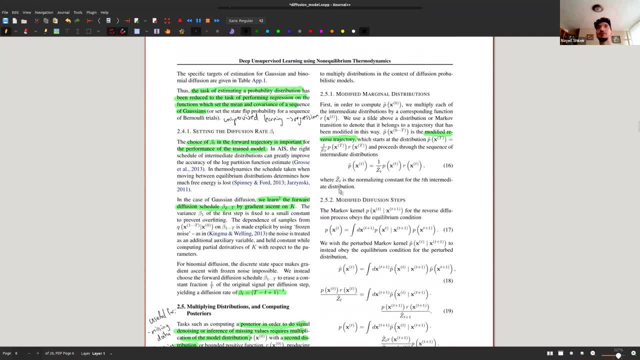 sort of get your normalizing, normalization constant, which before was sort of very intractable to sort of calculate, you're able to sort of compute this much easier compared to other generative models. Yeah, and so sort of you modify your reverse trajectory which now starts as sort of this: 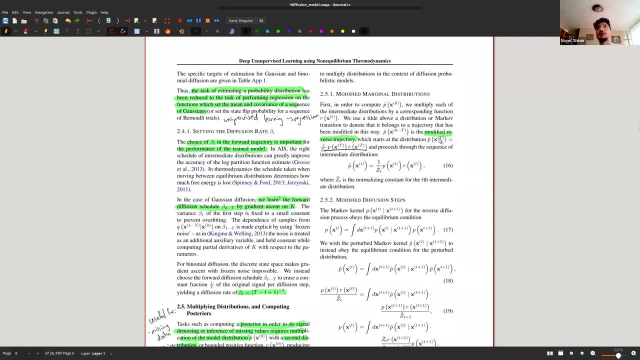 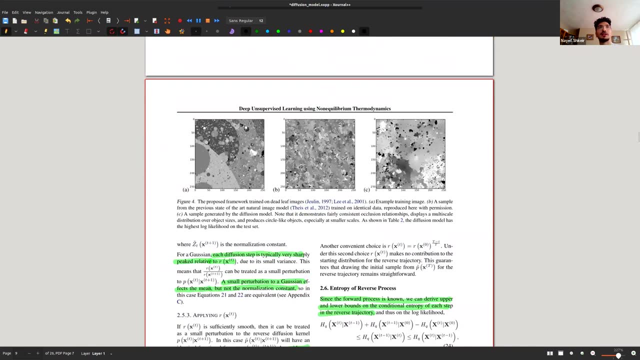 distribution, where this is a, where this p of xt is just a normal Gaussian, And so they do some. so this is not too important. I don't think I have time to go through this, but yeah. so, and at the end I say so for each, for a Gaussian, each diffusion step is typically 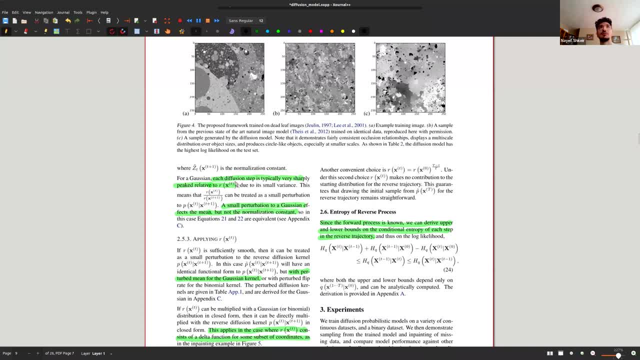 a very sharp peak relative to your probability distribution that you're multiplying by, And so because of, because of a small variance, and then you can treat this as a small perturbation. So that's basically the whole idea right. you have your diffusion process, your reverse process, 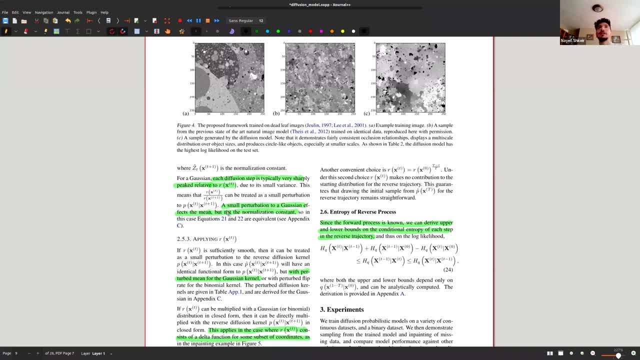 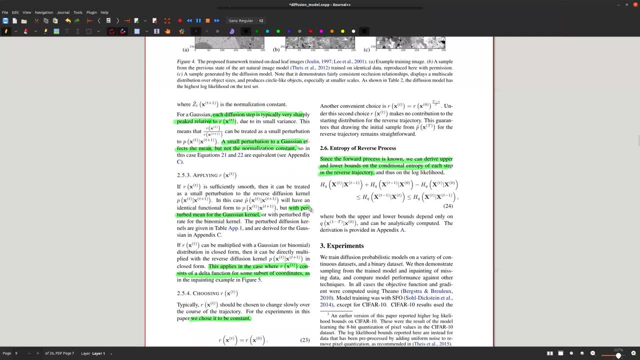 and you perturb it slightly to do sort of denoising or sort of filling in missing parts of an image? Does it also mean that if you completely reverse an encoding, so you you encode and then decode, then the decode itself is actually also a Gaussian distribution? just very, very, very. 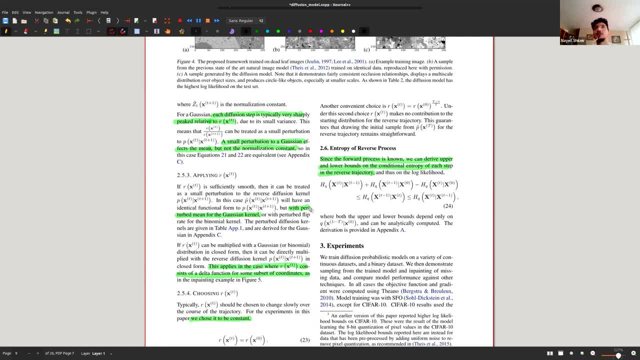 highly peaked. Yes, yeah, yeah and it's yeah, so it will be sort of like tiny, small Gaussian steps. Yeah, because the, the sigma, because it's of course the sigma is a function of the where in your trajectory you are. so so you would expect it. it sort of pulls it out. that's cool. 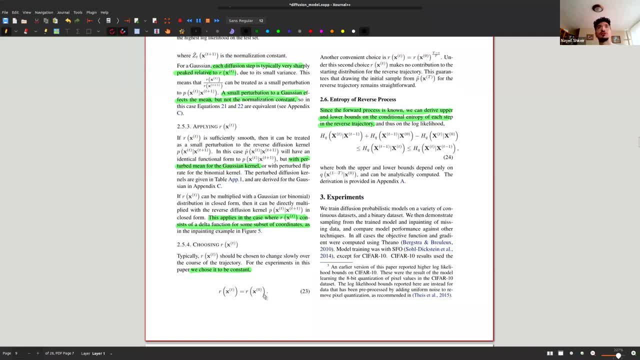 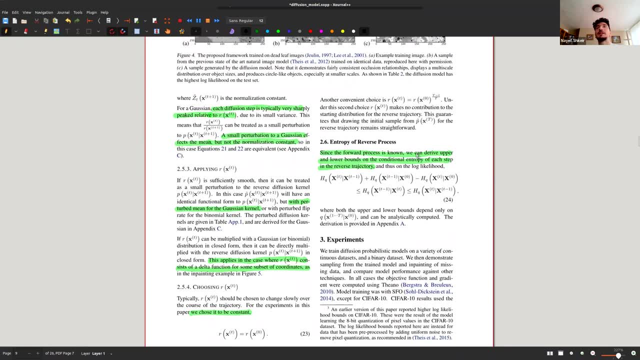 And yeah, and so then they say so they choose this distribution r to just be a constant In this case. so we choose it just for sort of convenience and then so they get, and then they can calculate sort of the entropy of the reverse process, and so, since the force process is known, we can derive an up and lower. 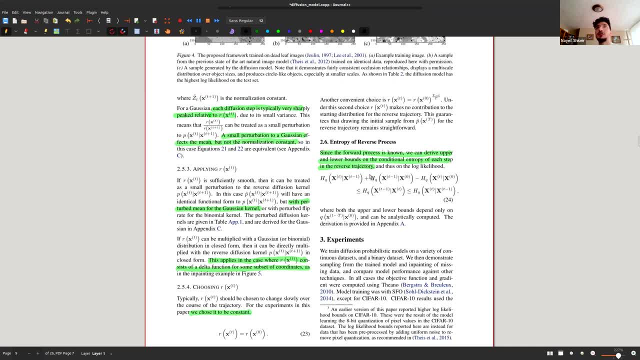 balance in the conditional entropy of each step in the reverse trajectory, Which is, I guess, super useful sort of like diagnostics and look likelihood estimation. But yeah, so that's pretty much The algorithm of diffusion models, and so they do a couple of experiments for results, so they test it. 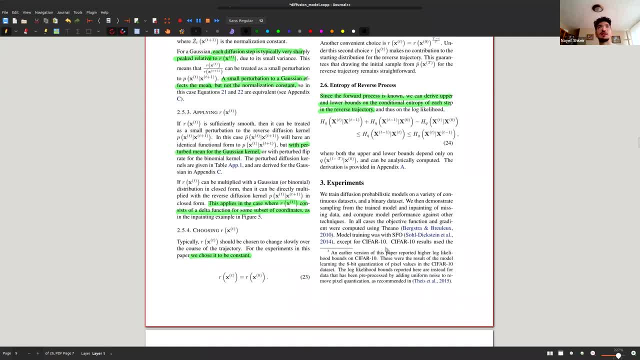 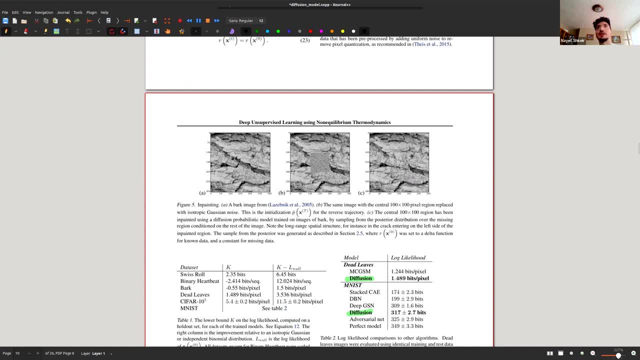 on the c410 data set. they do in painting, where they take this bark image and then they take a, I think, 100, 100 by 100, 100 by 100 by 100 pixel region and then they sort of just make that just full isotropic Gaussian noise and they push that through their version. 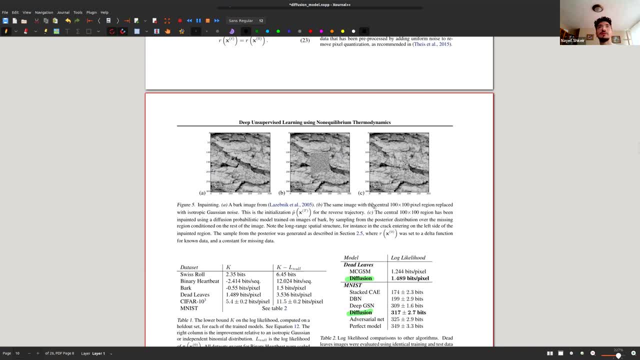 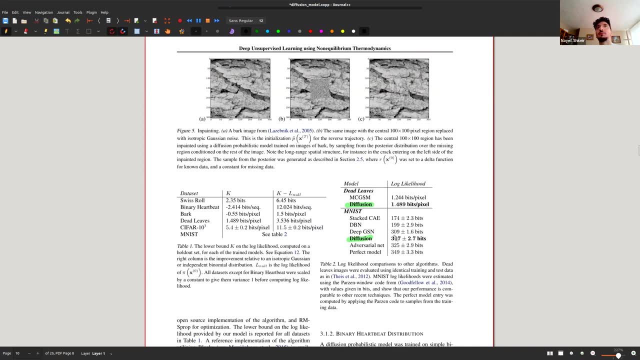 They do that in a sort of reverse process to sort of fill that region in Result wise. they sort of They did on par with other generative models, so Again did a bit better. I guess that's not really the problem, that an issue here is just more of the actual idea of 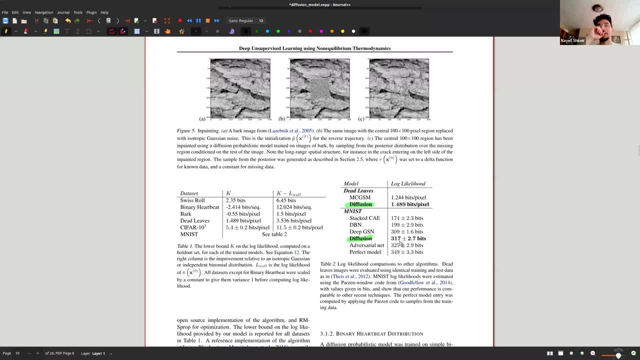 Whether they're not trying to sort of get the best Metrics for that. The problem, The problem, The issue here is just more of the actual idea. They're not trying to sort of get the best metrics for that. the papers that are getting sort of published right now. in the last couple years, the diffusion, 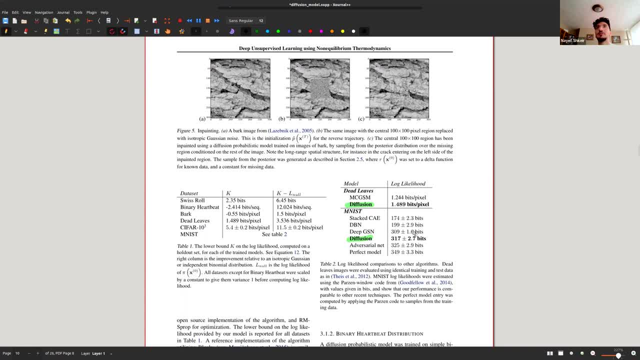 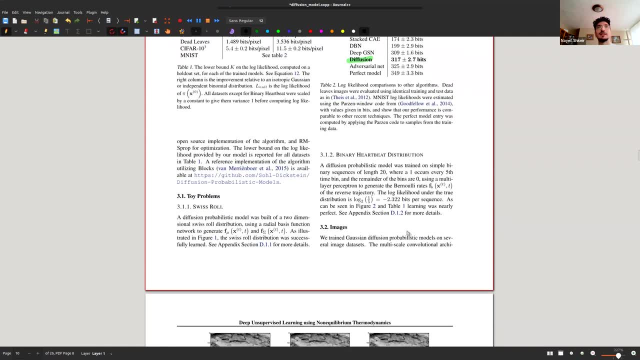 models have, like no other model have been, has been able to beat them in uh metrics, wise for image generation, uh, so so that's, that's pretty good. oh yeah and so yeah, and, like mentioned before, they do the swiss roll problem too. um, where? so you had to generate the mean and sigma. 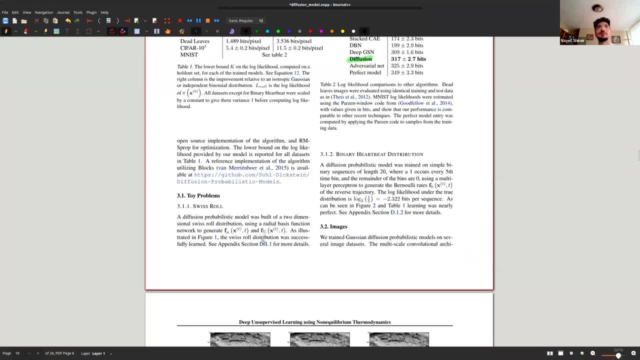 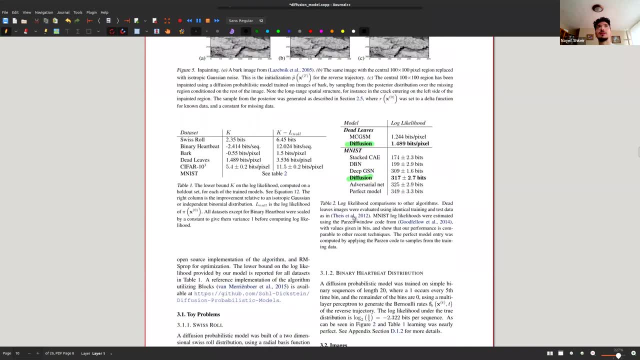 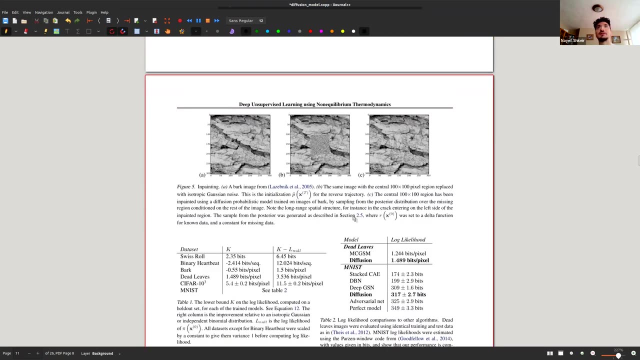 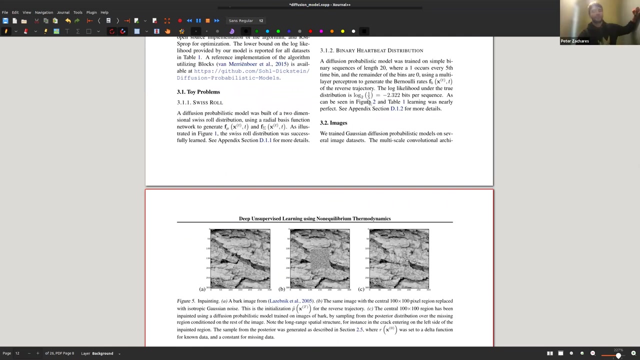 and it was sort of successfully learned. uh, and they do a binary example where they sort of generate, i think was the image for like heartbeats- no, i can't find it now, but yeah, so. yeah, so they do a binary problem as well, because, uh, well, yeah, could you keep going up? it's on the same pages as c part data. 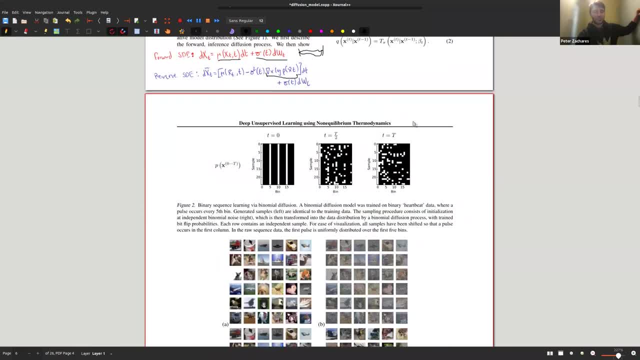 one thing i saw that with that and i was like there's something fishy here for me is that, um, so this is heartbeat data and the, the, the final distribution that you're diffusing to is just random, uh, independent noise on binary noise on each pixel, yeah, um, but the. 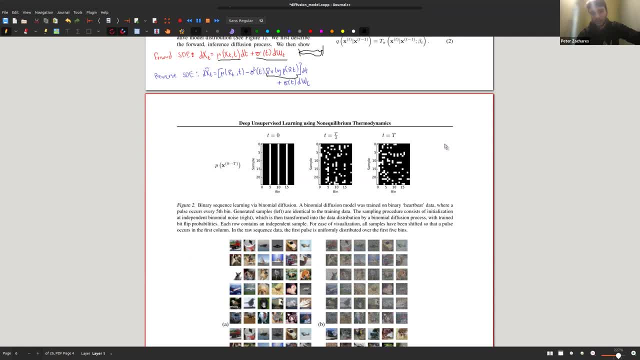 first column that is mapped to is all white, which is highly improbable. so i was thinking, yeah, that doesn't make sense in terms of, like the mapping from the heartbeat, the structured data, to the other. okay, yes, it's because, so they say, for ease of visualization. that's why they put it. so all samples have been. 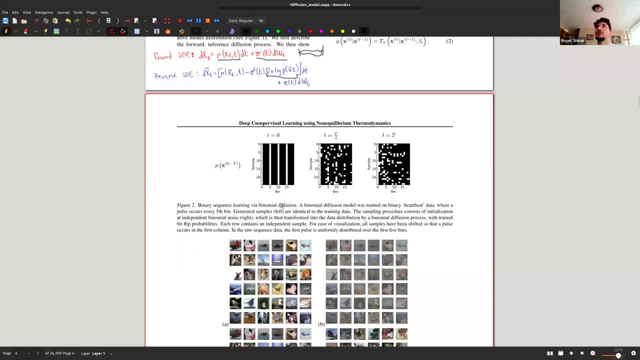 shifted so that a pulse occurs in the first column. so there's always going to be a pulse in the first column, but i don't understand why it maps to having a pulse in the first column. maybe i guess they keep that. they keep that, uh, uh. so they, they keep that there, right, they don't modify. 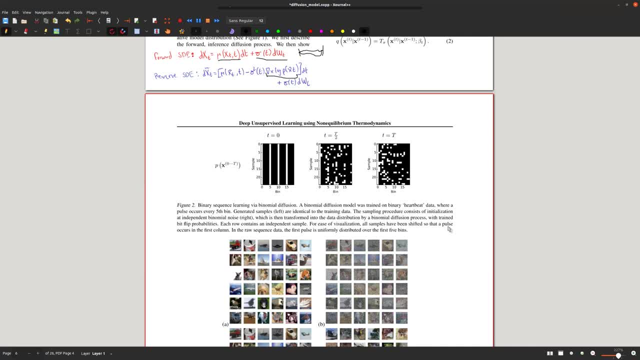 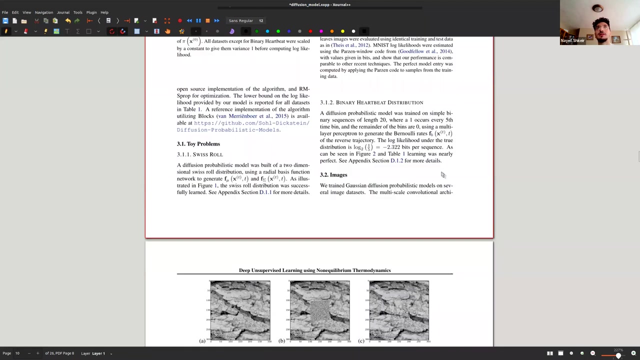 when you, when you reconstruct the last image, you probably get something that looks like the first image, but but possibly shifted, and and by by keeping the first one, they essentially forced the backwards process to always start with the period at zero. essentially okay, thanks, um, yeah, okay. so these are yeah. so they did the binary uh problem. they did the cifar data set. 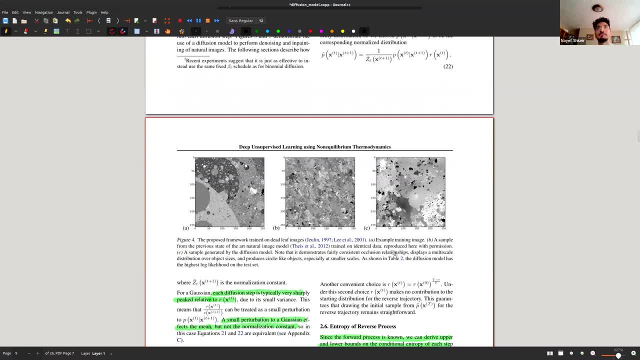 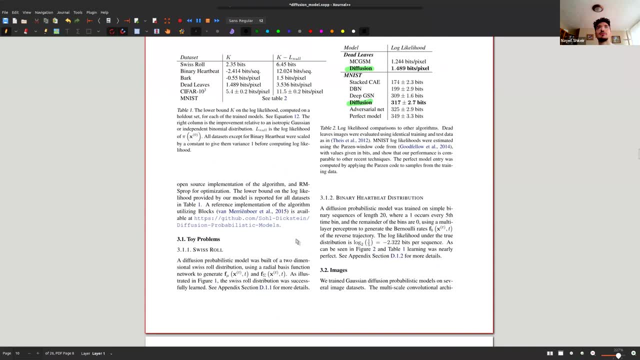 and they did image in painting and um this one was yeah one on deadly fish. and they did image in painting and um this one was yeah one on deadly fish. and they did image in painting and um this one was yeah one on deadly fish. so they tested on sort of quite a lot of different data sets. 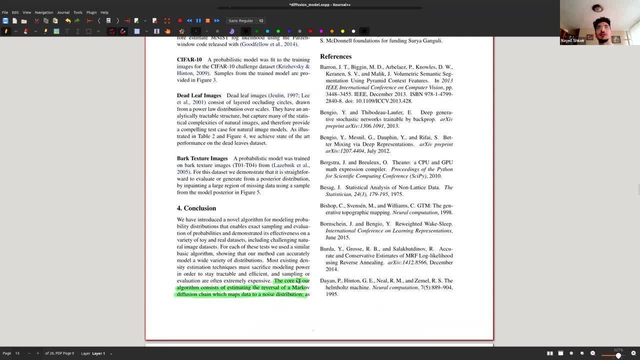 and yeah, and i think that's pretty much all and so, yeah, so to conclude, so the core of our algorithm consists of estimating the reversal of the mark of diffusion chain that maps data to a noise distribution, as the number of steps is made large, and so this algorithm can fit any data distribution. 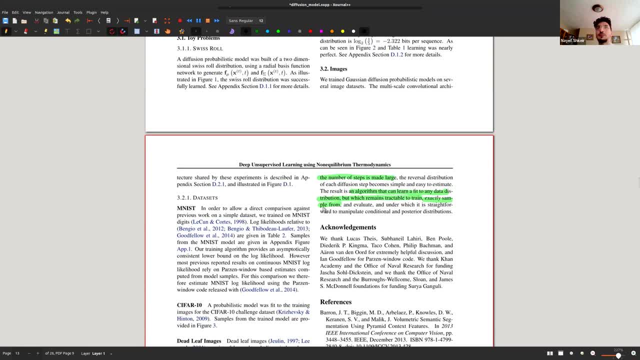 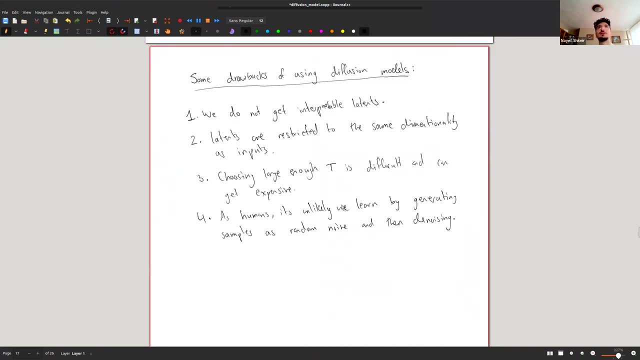 and it remains extractable and it can exactly sample. and you can exactly sample because, well, every step in your mark of change is exactly defined, uh, by your, uh by a gaussian, uh, yeah, so this is all sort of well and good, and i thought of sort of maybe mentioning some drawbacks. 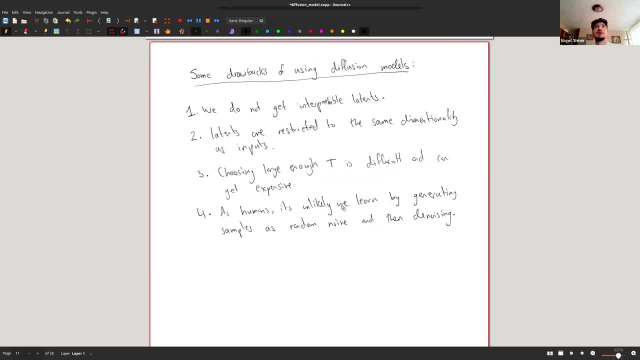 of these models before i answer only five minutes left. so some drawbacks is: we don't get interpretable latency. so usually with sort of these auto-encoded uh models, you take your distribution, you compress it to some lower dimensional latency space in the, in the hopes of like maybe getting some information from 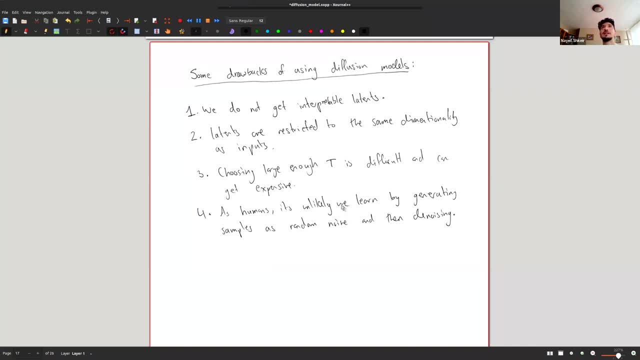 uh, this latent space about whatever distribution that you have. but here you don't really, you can't really interpret the, the latent representations. it's just your image plus some gaussian noise. uh, the latent is also restricted to the same dimensionality as the inputs, which can be a problem, especially if you want to do sort of image compression or compression problems. 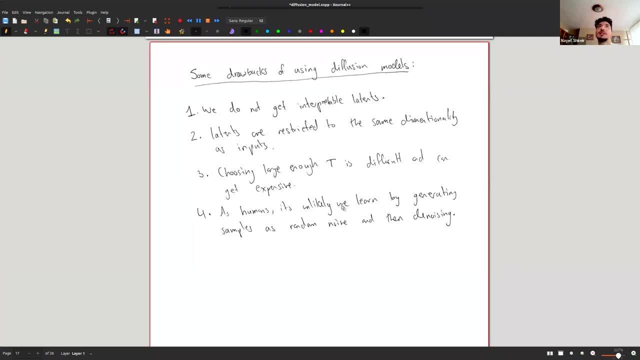 important part is. so choosing t large enough is difficult and can get expensive, because if you don't choose your t large enough, you're not going to be at isotropic Gaussian noise at the end, right. so you need to choose it such that you do end up at isotropic Gaussian, or close enough to 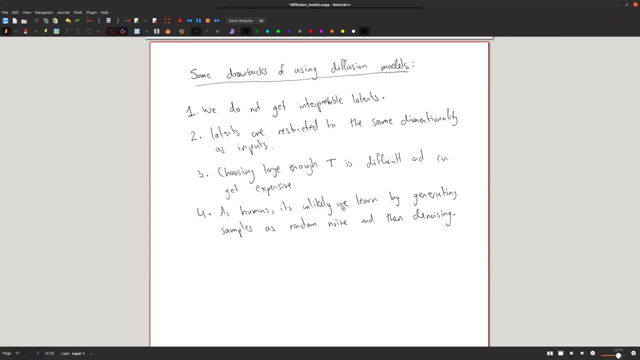 an isotropic Gaussian distribution. why is that actually important? isn't actually more the number of steps you take, like, like the you would think that it works better. the the fewer input noise you, you, you add at each step right, so you learn less right? that's the the idea of here is it's like 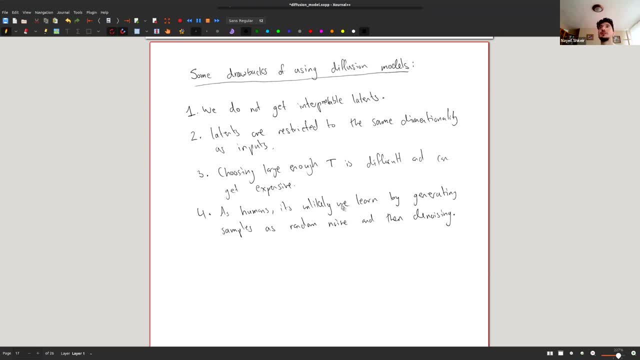 you try to do sort of tiny incremental changes so you can learn as much as you can. yeah, so as you tend to an isotropic Gaussian? yes, but but why does it matter that the last image is indeed isotropic? if you don't have an isotropic option at the end, then your analytical computations that you 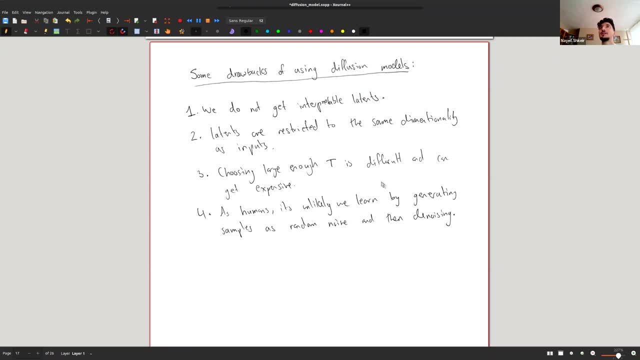 did at the top aren't going to work out, they're not going to end up being as nice. so that that's. that's a problem there again. that brings me to the to my, my caveat at the beginning, that they don't quite understand whether it would be truly isotropic. on on, on each, for each individual image. 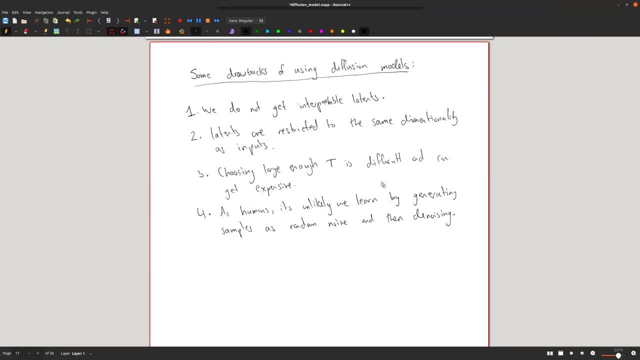 do I get isotropic or isotropic? isotropic Gaussian noise out At the end? yeah, you get fully, mean zero covariance, identity. Yeah, And that is the same for two different images, right? Yes, yeah, Yeah, then I still don't understand. 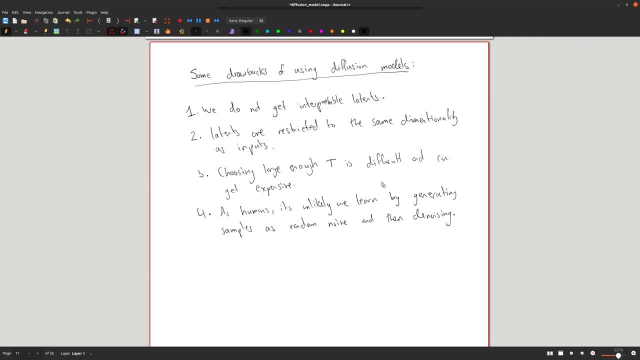 how possibly we could reconstruct anything from that, even by restricting ourselves purely to Gaussian. I don't think that it almost looks like it's a very, very good image like denoising, where it essentially makes use of structure information. that is maybe not. 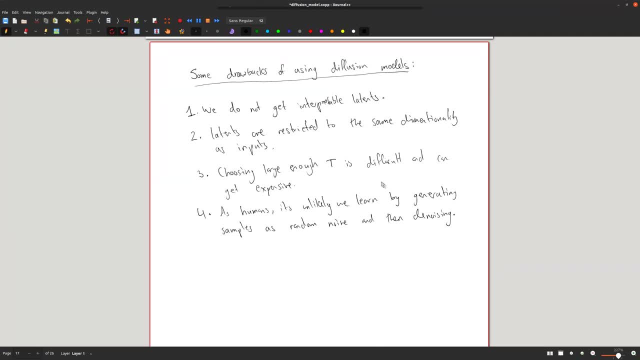 visible by eye, Because we might be able to see that structure in these noisy, grainy images, but it's still there And it gets amplified and put into something that looks very reasonable because it makes use of the prior that is then being learned by the process. 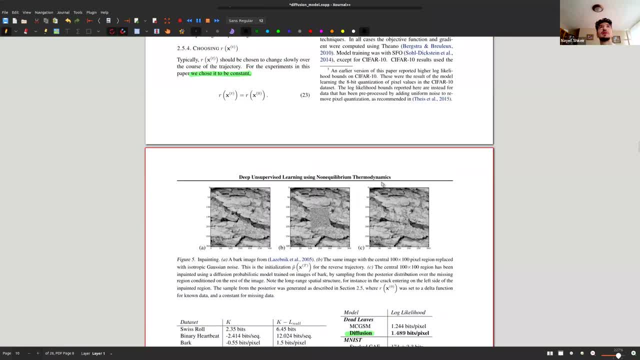 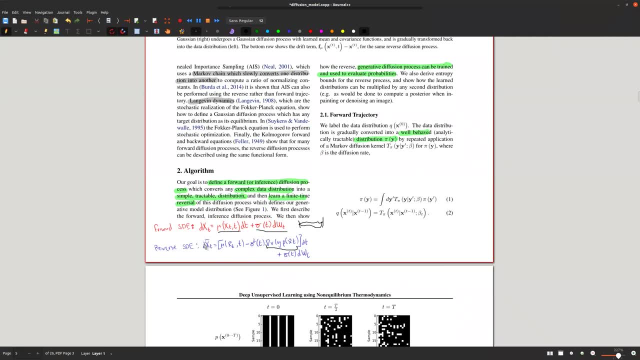 But I feel to be. Maybe it would be easier if you think in this sort of estimate, Right? so you're saying that the initial condition, the initial condition x, tilde, is going to be an isotropic Gaussian right. So it's just going to be some isotropic Gaussian variable. 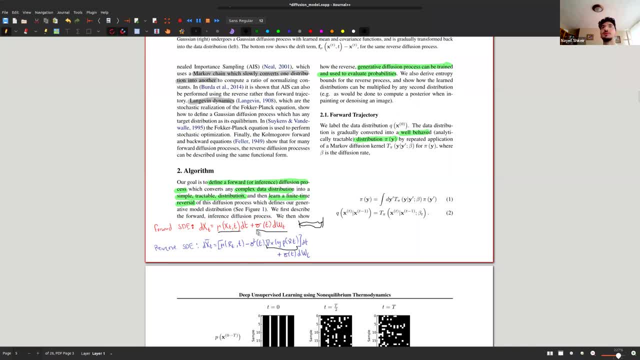 And then you modify that based on your mu and your sigma that you've learned. Yes, but mu is a function of that isotropic Gaussian right, Yeah, but not sigma. But sigma is only a function of time, right, So it doesn't contain any information that possibly could. 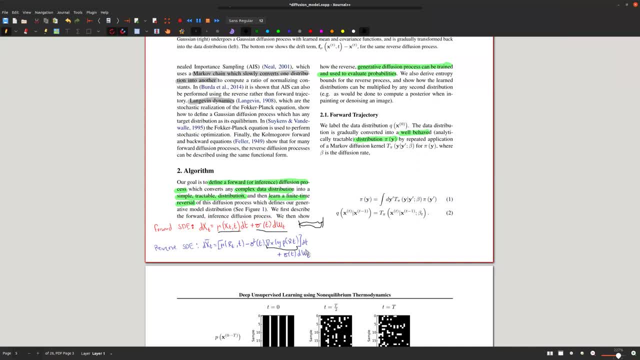 help me differentiate between different like images. yeah, Yeah, But all of the functions that you're learning, they're not. they don't take parameters in as an input, They take samples in, So they're not like nothing's a function. 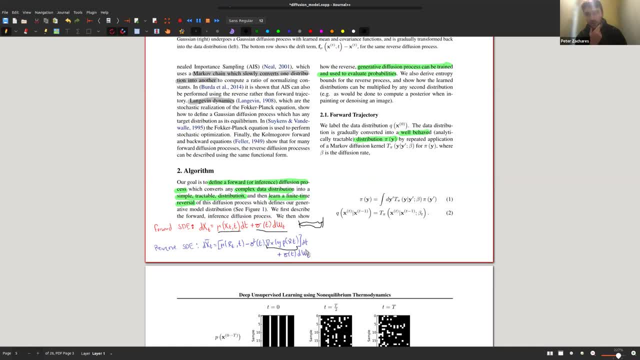 of the isotropic Gaussian. It's a function of a sample from the isotropic Gaussian. Wouldn't you expect that the? I would have thought that the point was that the exact piece of the problem in the picture at the end is essentially a Gaussian noise. 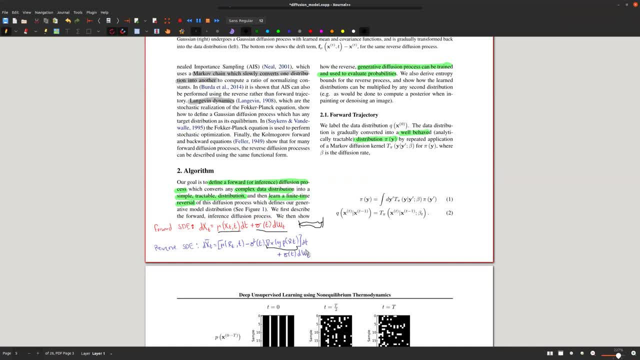 It is yeah. And so that means if I reverse from the very last step, if I take this SDE at the very last step, it would look the same for two different images because it would be the same. So how could they possibly, if mu is only a function of? 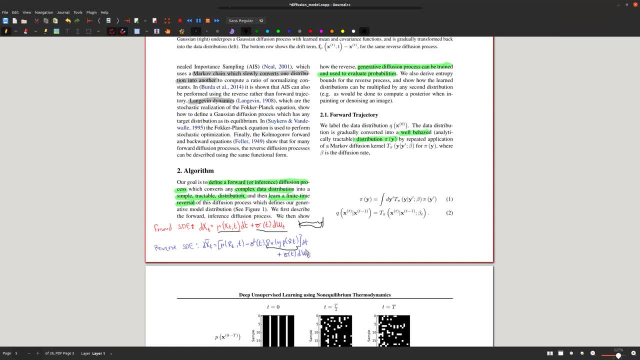 is also Markovian. how can it possibly, how can the solution of this equation possibly diverge? but if, Yeah, I mean I don't think it's going to be the same for two different outputs, For that case I think I'll need to sort of go into a little bit of detail. 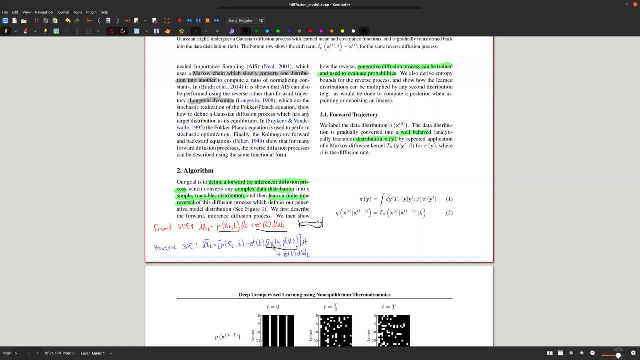 but this is a gradient over the data that you have which isn't then going. it's not a gradient over your isotropic Gaussian. OK, OK, Yeah, So I think it would be good if I go, if I do sort of paper. 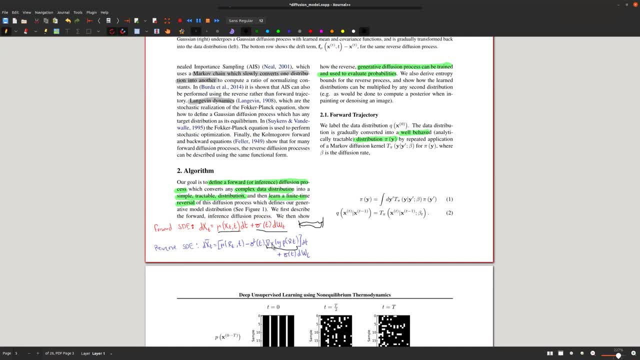 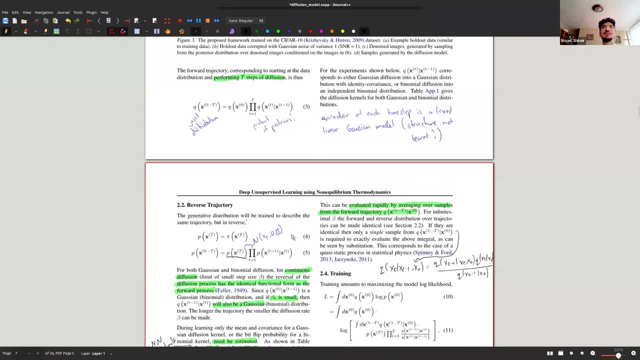 in the next couple of weeks. that goes into sort of this model that I've been working on. Yeah, It'll be a little bit easier to understand. That would probably be a good example. yeah, Yeah, Yeah, This notation was. it was a bit annoying for me. 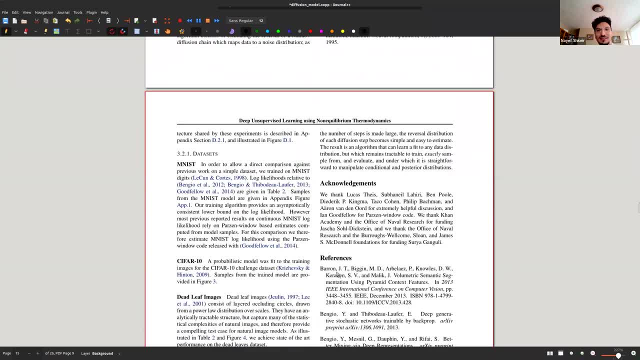 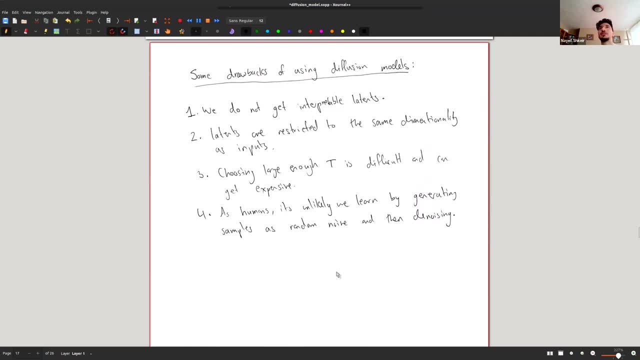 It didn't explain much, but yeah, it's OK. Oh, and I guess the time's up. but one last drawback is: as humans, it's unlikely we learn by generating samples. We generate sample as a random noise and then denoising right. 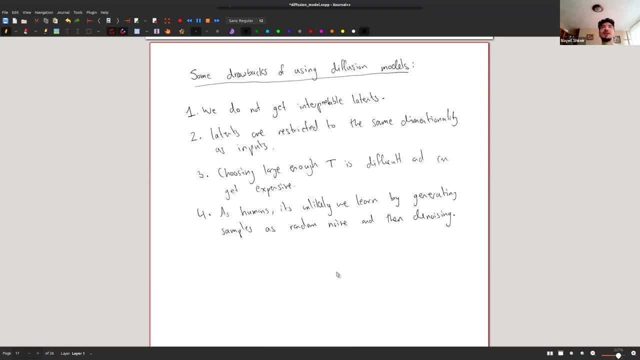 So it's. it's sort of- we're trying to sort of- model the way that humans learn, And I don't feel like this is the way that humans do actually learn. So, but it's a very good model though and it works very well.